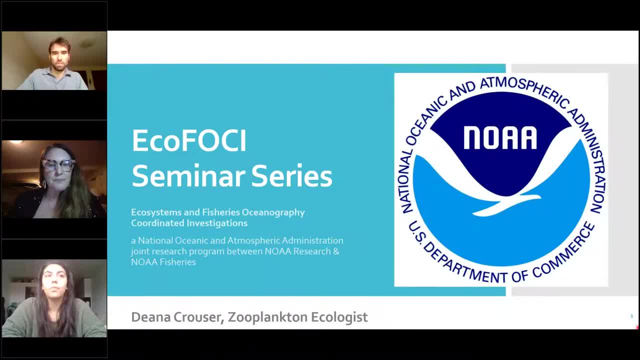 wwwecofocinoaagov. And again we sincerely thank you guys for joining us today for this season as we continue kind of this all-virtual seminar series. This is the last talk this season and our speaker lineup coming up can be found always by the One NOAA Science Seminar Series. 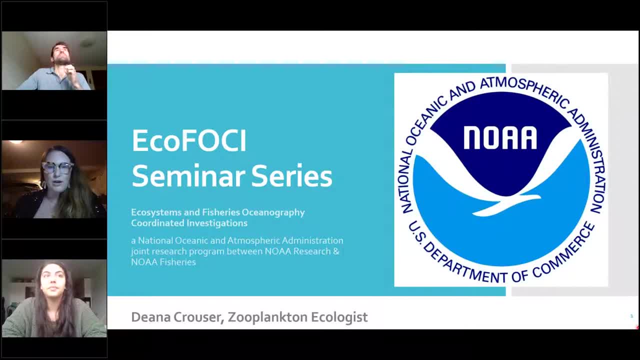 on the NOAA PMEL calendar of events. We are here Wednesdays at 10 am and we should be beginning probably March 3rd, so look for details forthcoming in the new year. Please double check that your microphones are muted, that you are not on video, and then, during the talk, please feel free to type. 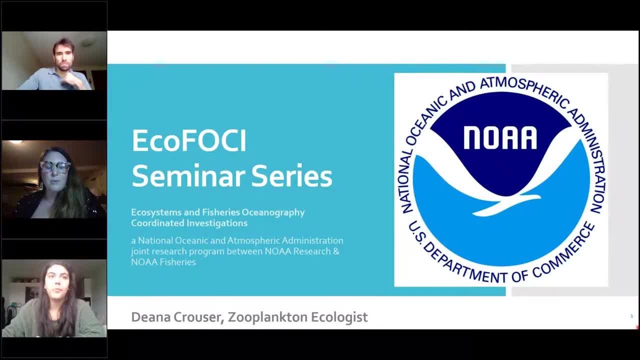 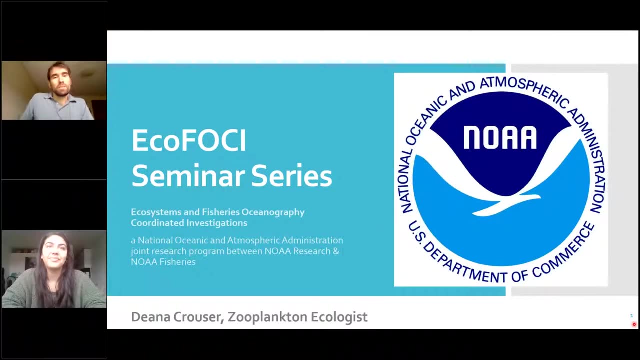 your questions into the chat. Both Jens and I will be monitoring that and we'll address those at the end of the talks And I'm going to hand this over to Jens and he's going to introduce and lead seminar today. Jens, all you, Thank you, Heather, Thank you everyone. 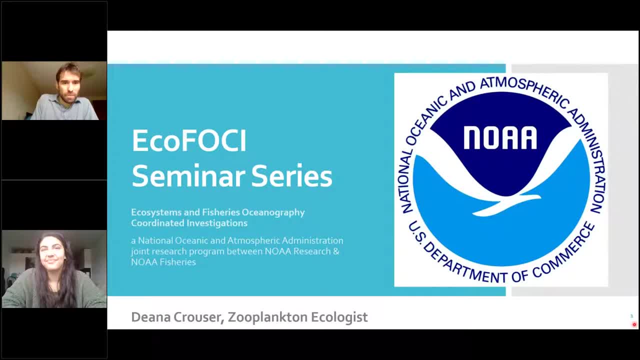 for joining in. It's a pleasure to introduce Deanna Krauser. Deanna is a zooplankton ecologist in our EcoFOCI group and she has a variety of projects focused on zooplankton identification quality assessment. She works on the chlorophyll analyses and data analyses of those data. 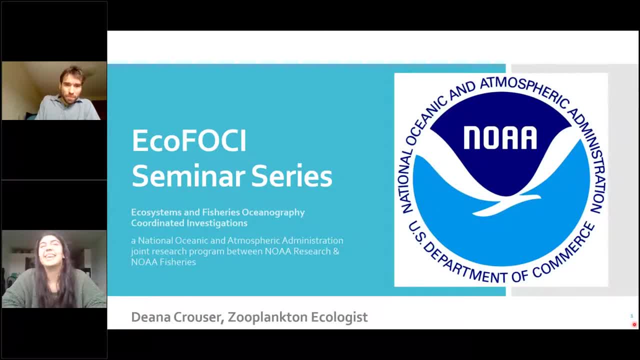 She also knows three to four different programming languages, which is very helpful when you happen to be her office mate, And lately she's been leading the group's zooplankton imaging efforts, which I think we'll hear a little bit more about today. 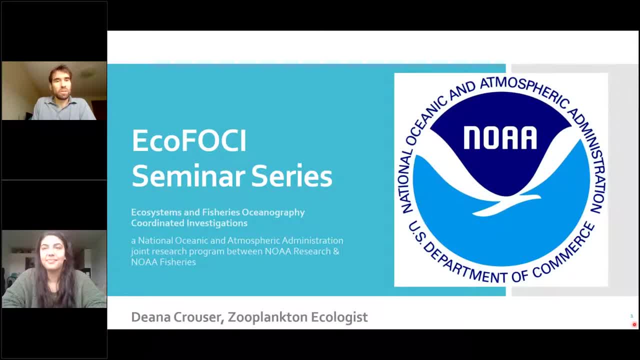 which is really, really cool work. Deanna holds a degree in oceanography from University of Washington and she did her thesis work with Julie Keister and Daniel Grombaum and researched the effect of low oxygen levels and ocean acidification on copepod cells, And she's been working on. 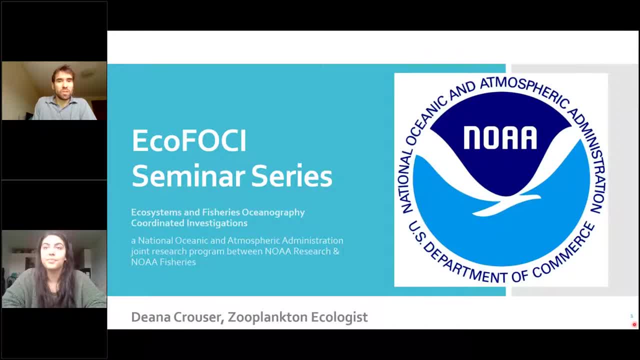 science distributions, And I'm going to swing it over to you, Deanna, right now, because I know you're going to talk about that. So go ahead. The floor is yours. Thank you, Jens. Hi, as Deanna said, I'm Deanna Krauser. I'm a zooplankton ecologist here at NOAA. Today I'm going to talk. 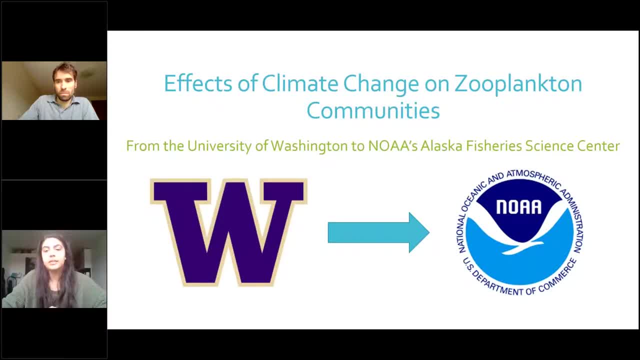 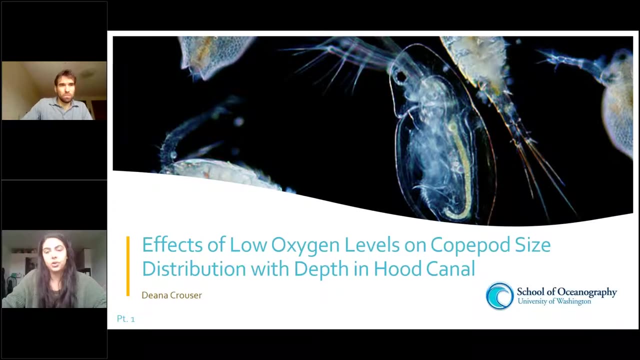 to you about the effects of climate change on zooplankton communities, from my undergraduate research at the University of Washington To my current work here at NOAA's Alaska Fisheries Science Center. So, as Jens said, I graduated from University of Washington with my BS in oceanography in 2019.. And for the first portion of this seminar, 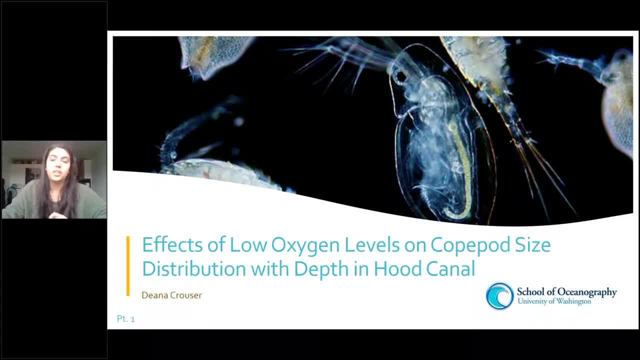 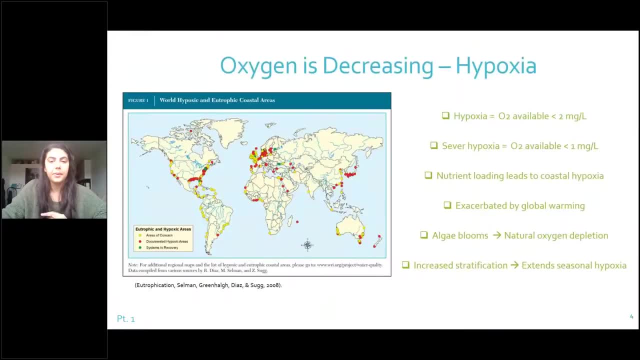 I'm going to present my undergraduate senior thesis, which investigated the effects of low oxygen levels on copepod size distribution with depth and hood. canal. Hypoxia, a condition in the coastal system, is a global warming. In fact, there's a decrease in the concentration of oxygen availability below two milligrams per liter. 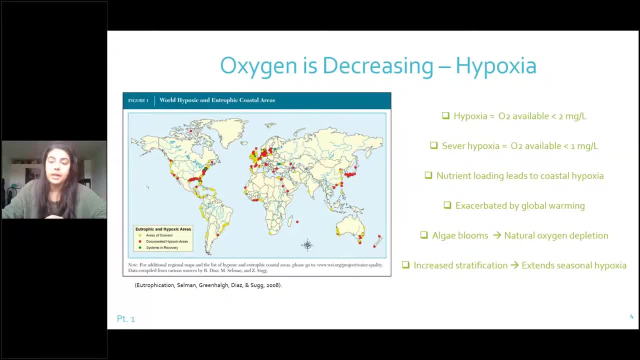 Incidences of coastal hypoxia due to changes in nutrient loading have steadily been increasing over the years. According to recent studies, 415 oxygen depleted coastal systems have been identified worldwide. This condition is exacerbated by global warming Through increased stratification and warming waters. Many coastal areas experience seasonal hypoxia due to high primary production as well as stratification, which naturally leads to oxygen. 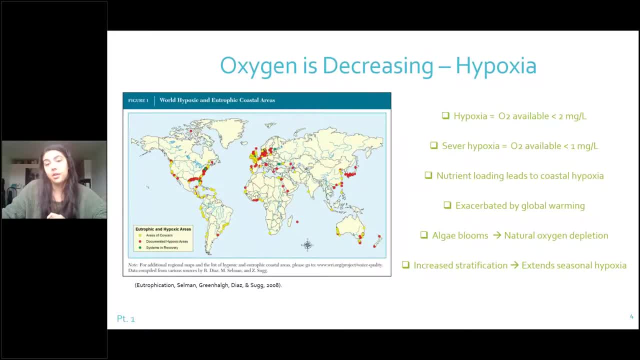 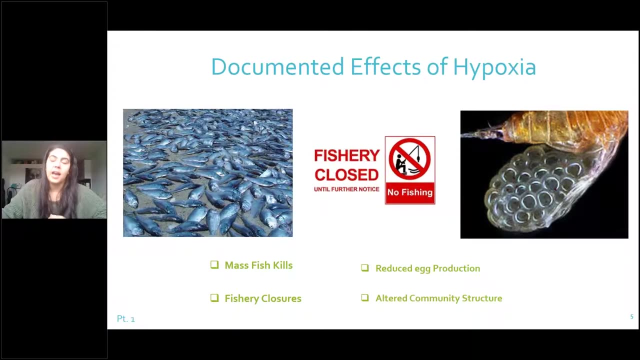 depletion, as algal blooms decay in late summer and autumn. However, the increase in the strength of stratification promoted through global warming is extending the length of seasonal hypoxia. It has been documented that hypoxic events can lead to mass fish kills and fishery closures. 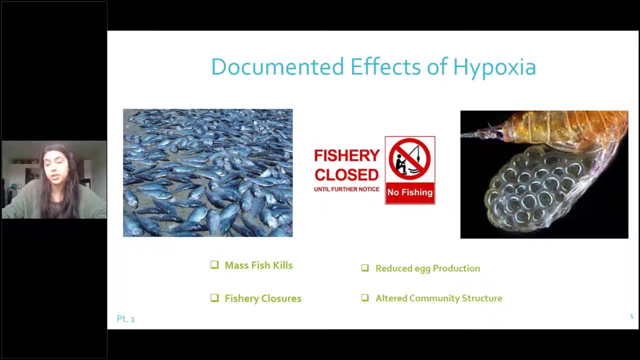 However, subtler effects of hypoxia are reduced egg production of copper pods, Altered community structure of mesozooplankton and hood canal has also been documented, A change which will likely affect the amount of energy transfer between trophic levels in the marine web. 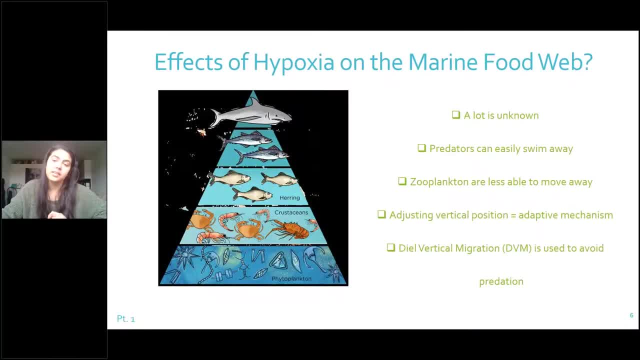 Turns out it is subtler and different depending on the cantilever Solium-Dιο and, if that's slightly underwater, knowcas включated. Fortunately, a lot is unknown about how hypoxia affects each aspect of the marine web. 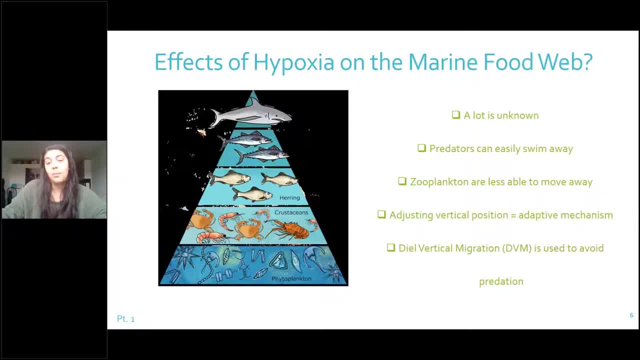 Predators like fish can deal with the extension of seasonal hypoxic conditions by simply changing migration habits and avoiding low oxygen areas. However, drifting organisms like copepods pay a higher cost to exploit adaptive mechanisms that allow them to better deal with low oxygen conditions. 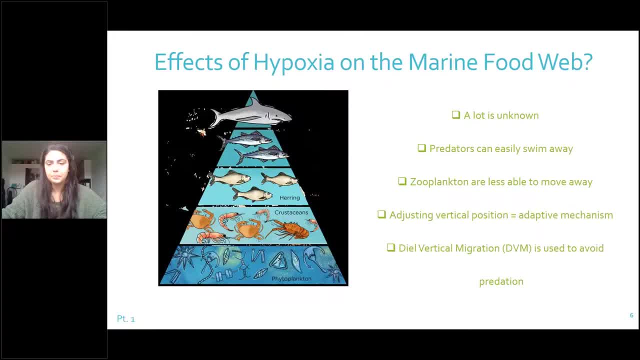 because they're less able to move away from affected areas. One adaptation of copepods is to adjust their vertical position within the water column. An example of this adjustment is dial vertical migration, when copepods occupy depths during the day and migrate to the surface to feed at night. 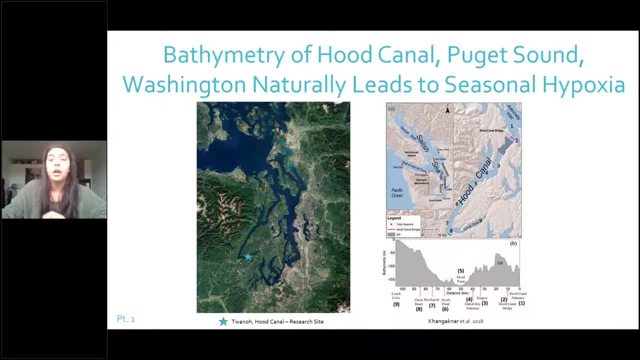 Hypoxic conditions occur seasonally in Hood Canal, a sub basin of Puget Sound, Washington, making it a good place to study the effects of hypoxia. Hood Canal is a deep and narrow basin that makes up the entire western branch of Puget Sound. 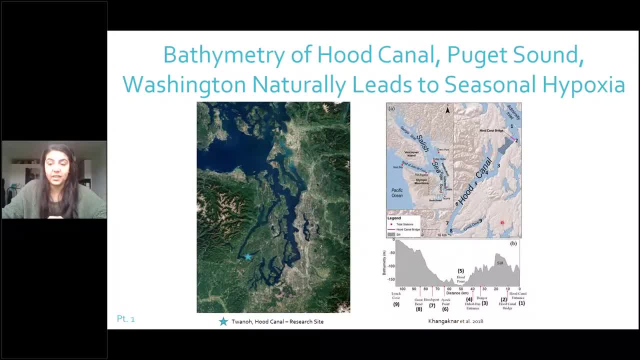 At the northern end of Hood Canal there is a long sill which limits ocean exchange and seasonally affects hypoxia. In the fall, tidal intrusions bring in dense waters that sweep over the sill and flow into the basin. Stratification occurs as this cold and dense water 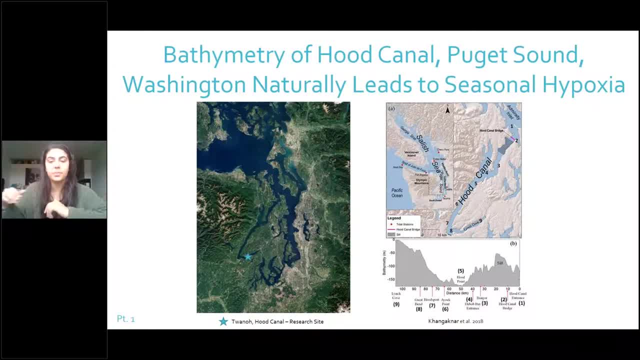 sinks to the bottom of the basin and then displaces the less dense bottom water towards the surface of the water column. This displaced water, which is low in oxygen concentrations due to respiration and a lack of mixing, leads to a mid-water layer of hypoxic conditions. 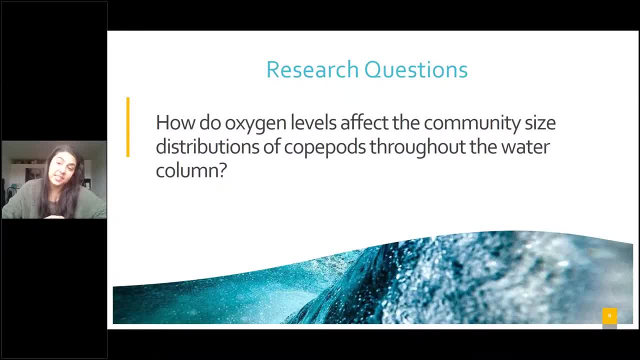 So the question I explicitly asked for this study is that: how can we reduce the risk of hypoxia? So the question I explicitly asked for this study is that: how can we reduce the risk of hypoxia? So the question I explicitly asked for this study. 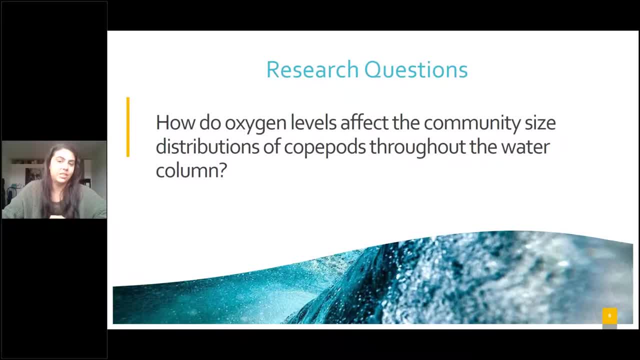 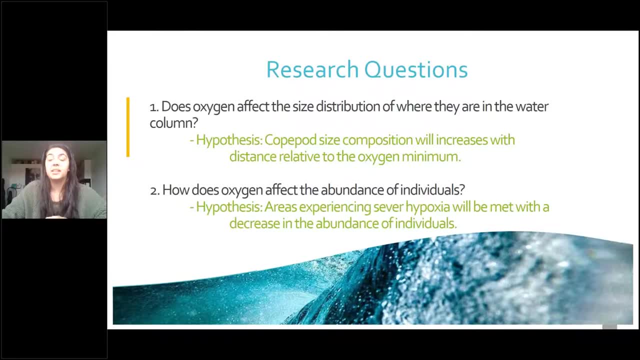 was: how do oxygen levels affect the community size distributions of copepods throughout the water column? And to answer this question, I need to determine two things. First, does oxygen affect the size distribution of where they are in the water column, Based on the theory that larger organisms 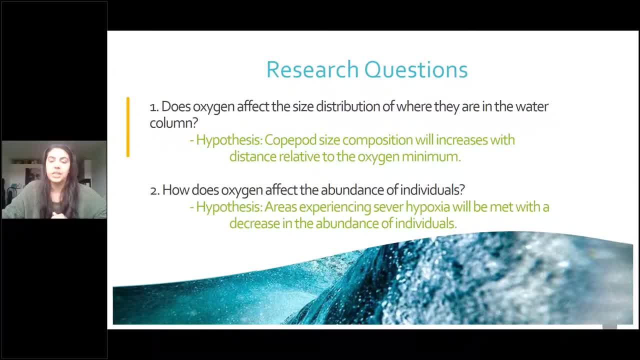 require more oxygen than smaller organisms to function. based on the theory that larger organisms require more oxygen than smaller organisms to function, I hypothesize that smaller organisms would well. I hypothesize that copepod size composition would increase with distance relative to the oxygen minimum. 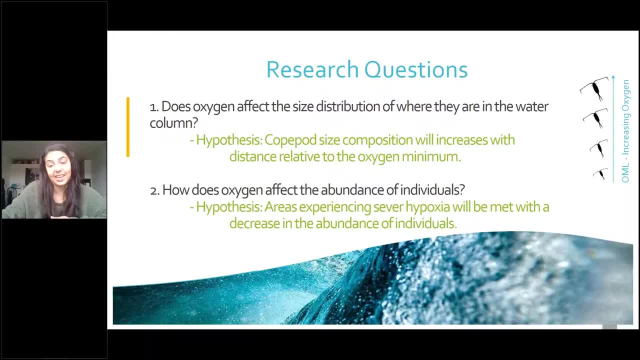 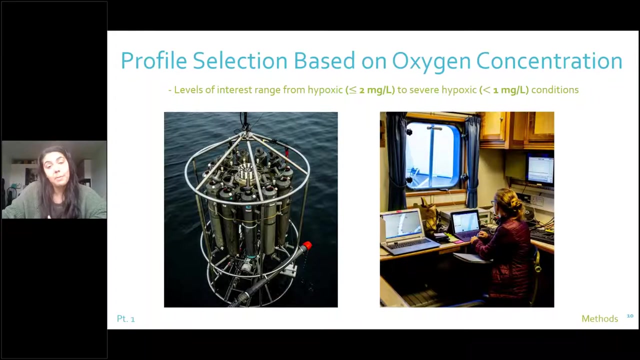 So something like this. And second, how does oxygen affect? how does oxygen affect the abundance of individuals If oxygen concentrations were severely low? if oxygen concentrations were severely low, I hypothesized that that's a good answer: a decrease in the abundance of individuals present. So, shifting into my method, section 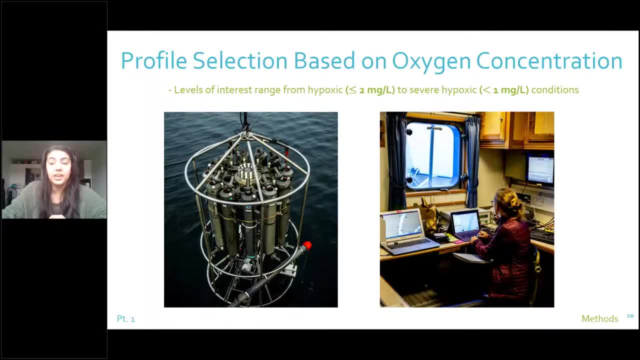 samples were collected at Tawano Hood Canal on the 19th of August 2017 and the 24th of September 2018. above the RV Rachel Carson, A CPD sensor fitted with an annually calibrated dissolved oxygen sensor was cast to determine target depths of interest. Profiles used in this study were: 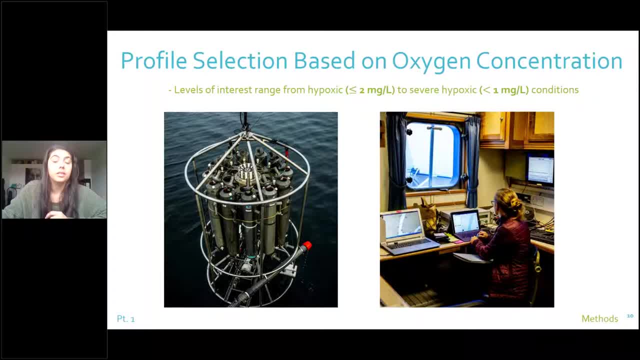 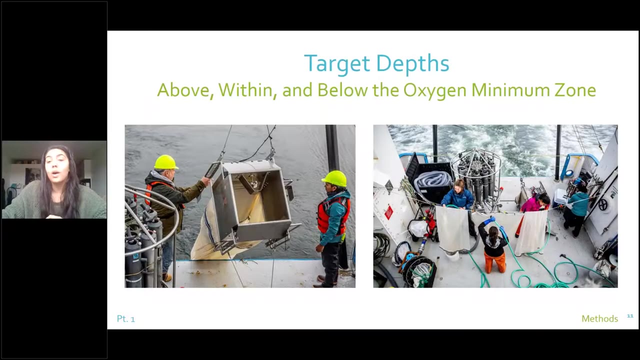 selected based on oxygen concentrations. Levels of interest range from hypoxic conditions- less than two milligrams per liter, to severe hypoxia, which is less than one milligram per liter, based on previous research conducted on copepod behavior under low oxygen levels. Once target depths were identified based on the obtained oxygen profile above, within and below. 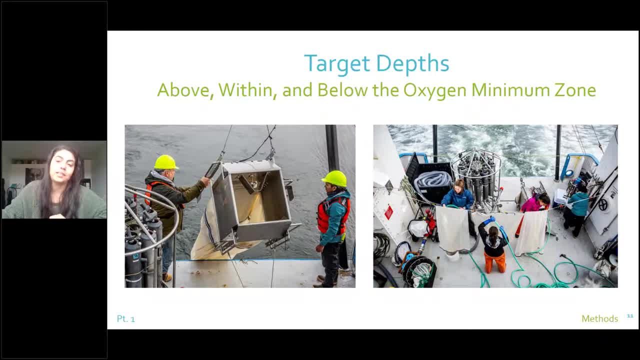 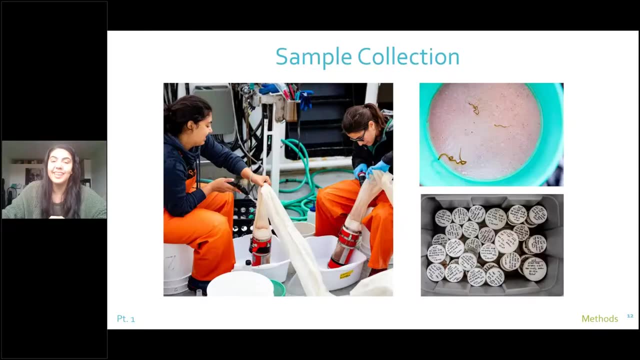 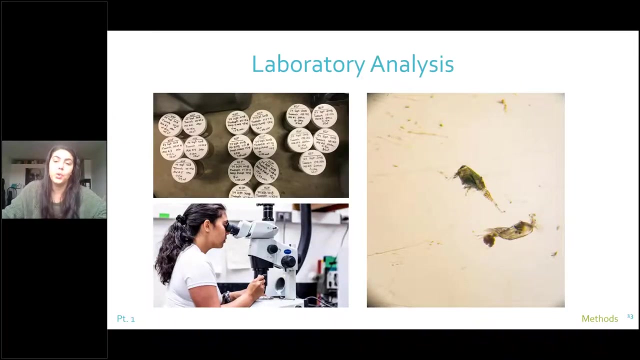 the oxygen minimum zone. oblique multinet toes were conducted day and night to observe diel vertical migration or DBM. Though plankton samples collected were preserved and returned to the laboratory for analysis, And in the laboratory, each zooplankton sample was quantitatively diluted and a subsample was taken for 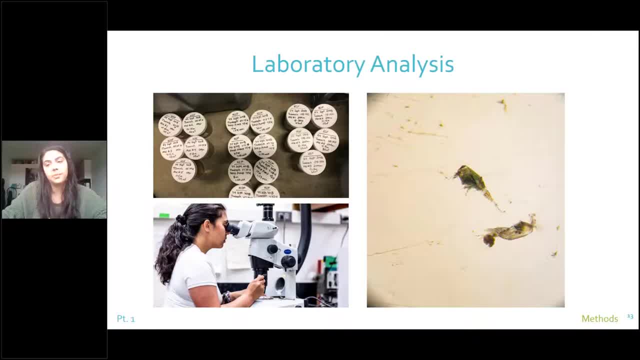 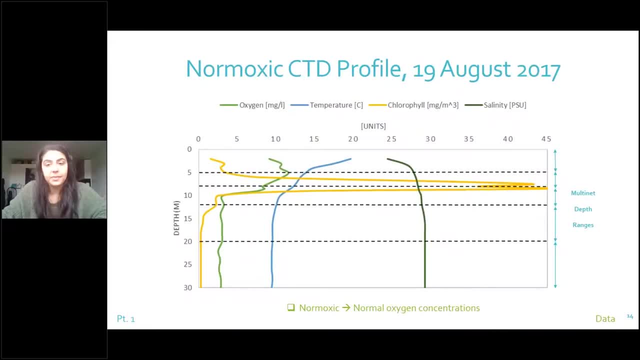 analysis, Each species of copepod within a subsample was counted and classified into five separate groups. Here is the CTD profile under normoxic conditions taken August 19th 2017 at 3: 30 am at Tawano Hood canal measuring oxygen. 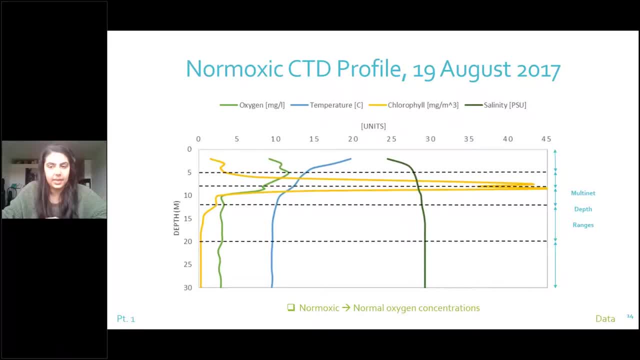 concentration, temperature, chlorophyll and salinity. The dashed lines here represent the depths and meters and the y-axis represents the well. the dashed line- sorry, the dashed lines- outline multi-net depth ranges and the y-axis represents the depth in meters and the x-axis 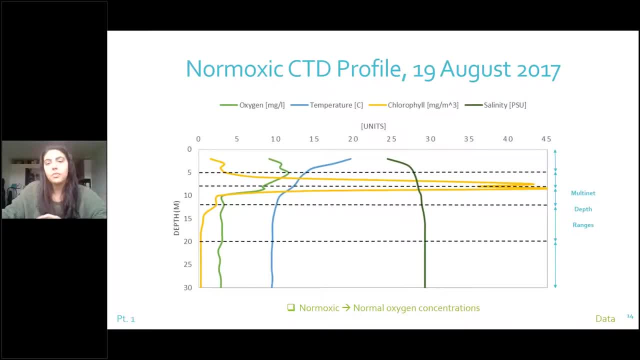 represents the depth in meters, and the x-axis represents the depth in meters. The dashed line here represents the respective units of conditions measured. Now, focusing on the oxygen profile represented by this green line, we can see that conditions never fell below two milligrams per liter, which is why we'll 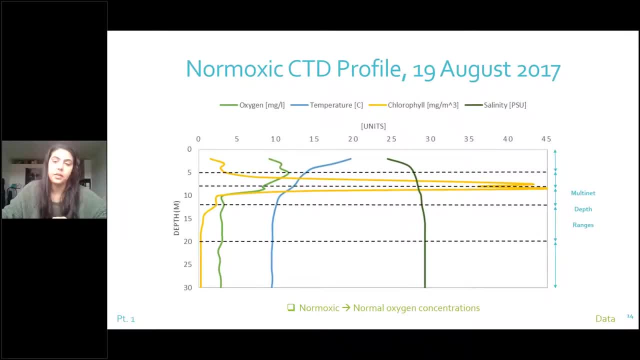 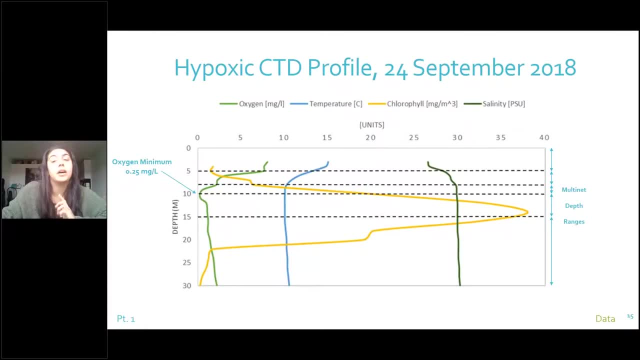 use this profile as the control. And here we have the CTD profile under hypoxic conditions. well, that was taken on September 24th 2018 at 6: 45 am. Focusing on the oxygen profile again, here in green we can see concentrations. 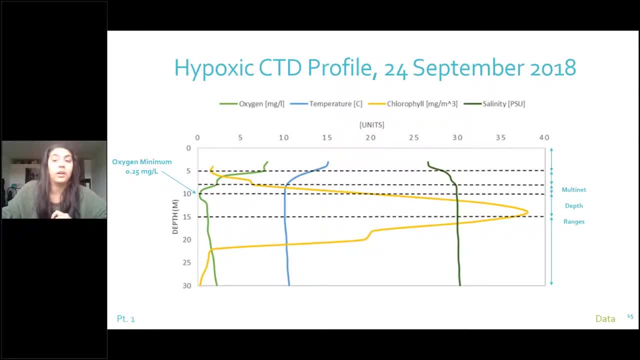 fell well below the hypoxic threshold of two milligrams per liter at the 10 meter. at 10 meters we actually observed the oxygen minimum level, where oxygen concentrations reached 0.25 milliliters milligrams per liter and making it severely hypoxic. conditions documented to significantly alter survival rates of copepods. 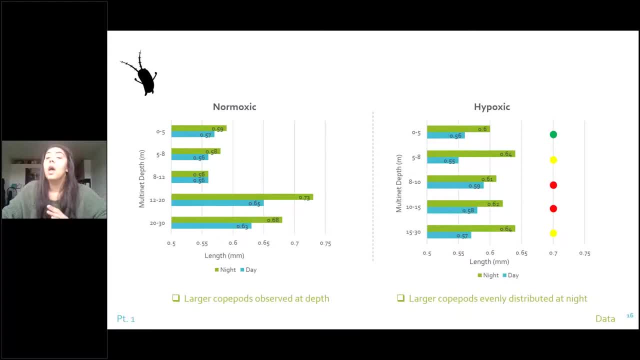 Now adjusting. my first question: does oxygen affect the size distribution of where they are in the water column? No, this is my size slide indicator. First we'll look at the distribution for the average size of the copepods under both normoxic and hypoxic conditions at night, which is depicted with the green bars. 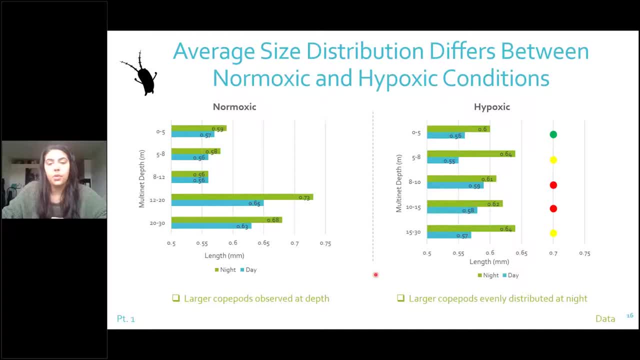 and during the day, which is depicted with the green bars, and during the day, which is depicted with the blue bars. The y-axis is the multi net depth ranges and meters, and the x-axis is the prozone length of the copepods in millimeters. Copepod size. 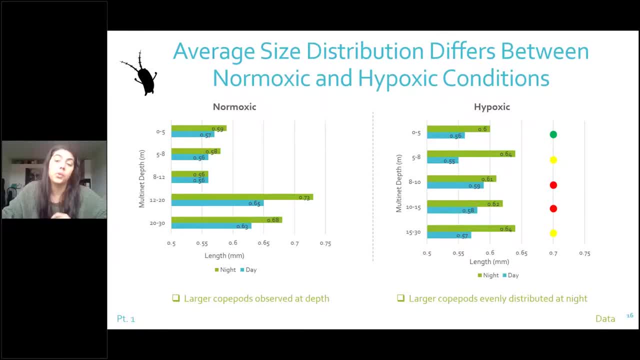 distribution significantly differed among depth strata under normoxic conditions- so this entire profile from 2017- as well as under hypoxic conditions, but only during the day. so just the blue bars in this graph. There were no statistically significant differences in size distribution among depths at night. 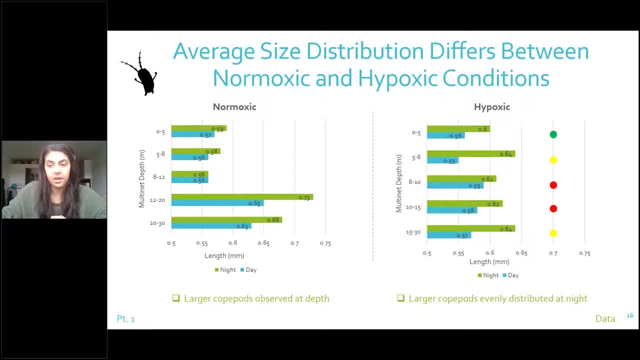 under hypoxic conditions. so that's the green bars in this graph. So we had a pretty even size distribution at night, unlike our normoxic profile. Note the green, yellow and red circles. these act as a reference and will be seen throughout my data to reflect normal, hypoxic and hypoxic conditions. 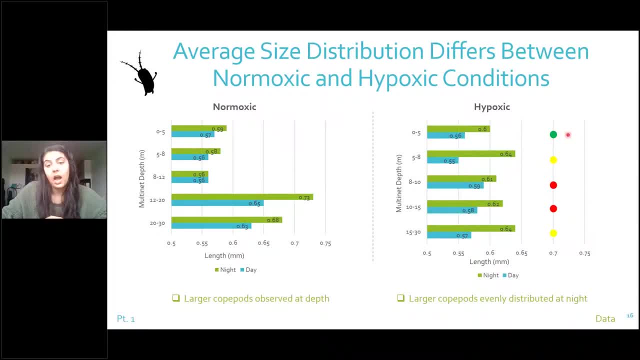 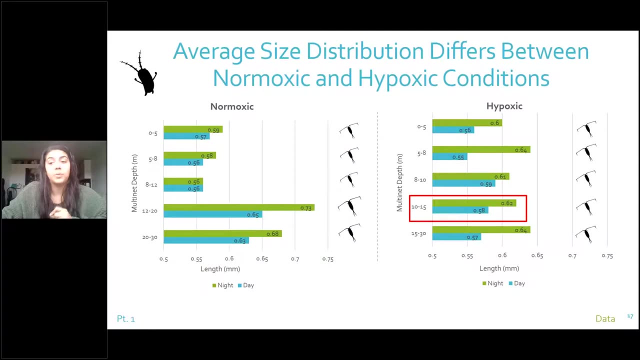 These act as a reference and will be seen throughout my data to reflect normal hypoxic and hypoxic conditions and severely hypoxic oxygen concentrations. The oxygen minimum of 0.25 milligrams per liter again occurred at 10 meters below the sea. surface And, on average, net two. the 10 to 15 meter range had the lowest oxygen concentration of 0.68 milligrams per liter, making it severely hypoxic- Recalling my original hypothesis- that I would find the smallest copepods occupying the oxygen minimum zone and size would then increase with distance relative to the oxygen minimum zone. this is where I expected to observe the smallest copepods at night. Stata did not support that hypothesis. I actually added these little copepods that are proportioned in size to kind of give you an idea of how much oxygen. 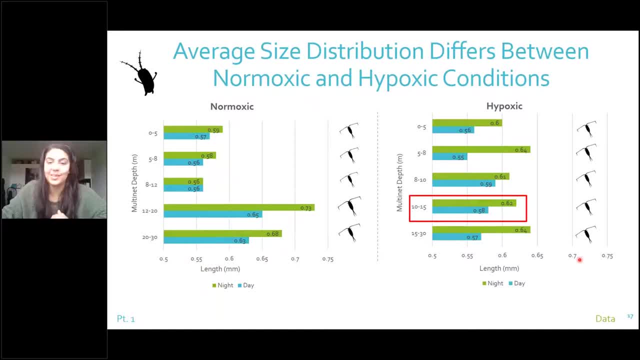 is in the water column So you can see these. it's really hard to distinguish the difference in size under hypoxic conditions And it's a little bit easier to tell that this copepod right here under normoxic conditions is largest and it kind of differs in size. So that's. 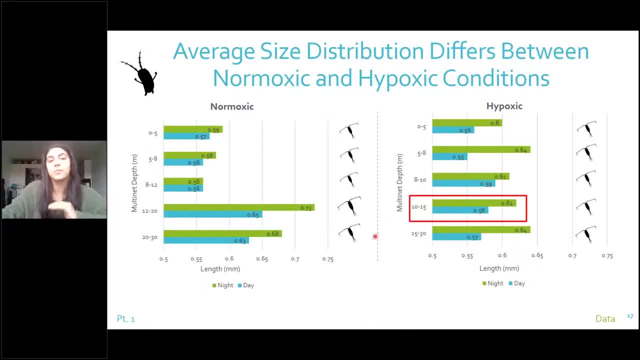 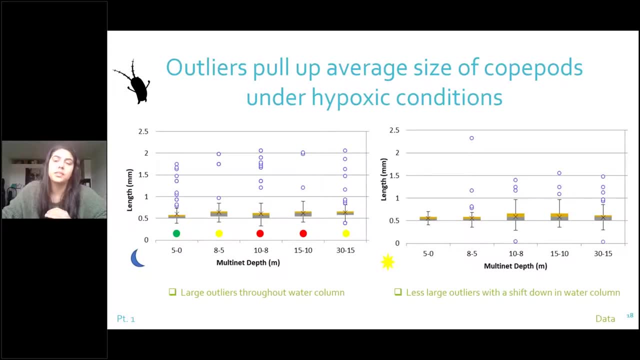 my statistically significant difference in size. when it comes to copepods in the water column, I used box plots. I used box to describe the size distribution of copepods throughout the water column and identify outliers within my data. Here we have box plots under hypoxic conditions at 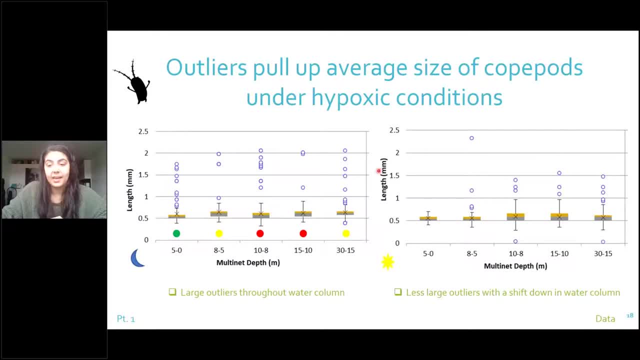 night and during the day. The y-axis is the prozone length of the copepods in millimeters and the x-axis is the multi-net depth ranges in meters. Under hypoxic conditions, numerous outliers are observed. If you have an outlier with a mass of about 90 milligrams per liter, then 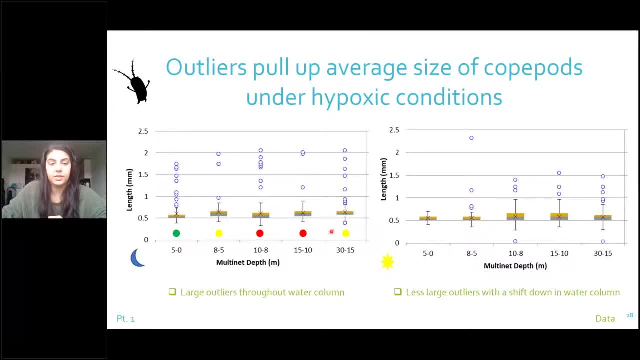 if you have a copepod that doesn't have the minimum length or the maximum amount of outliers, they low 찬 to a cost of about $1.. The mean value of length shown as the X's was drawn up the most by outliers in the surface. 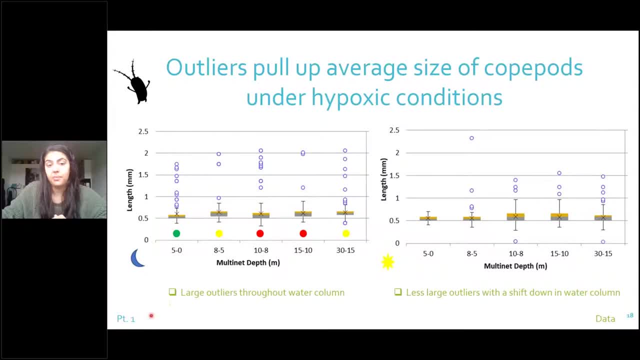 zero to five meters at night. so right here During the day, there was an overall decrease in the number of outliers observed, with larger copepods shifting down and out of the water. This is not a replacement for the amount of outliers. Some of the outliers are observed during the day, during the night, During the day there's 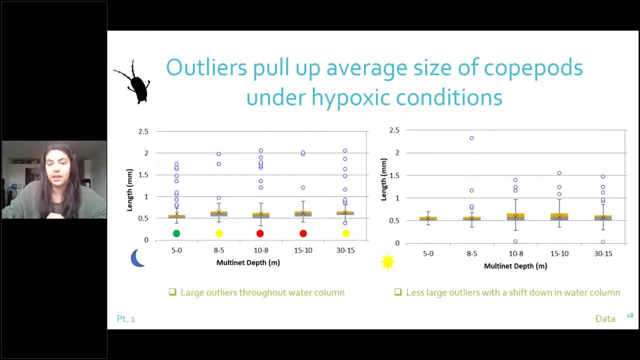 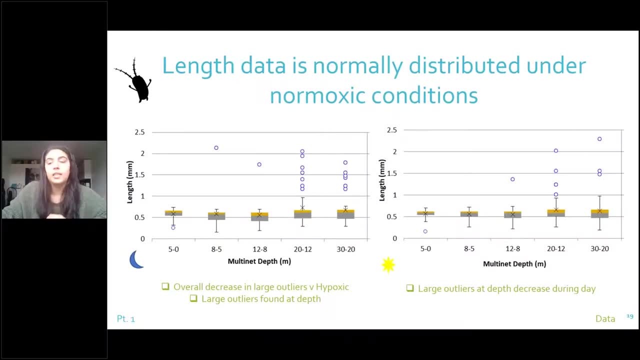 a decrease in the number of outliers observed, with larger copepods shifting down and out of the water the surface 0 to 5 meters during the day. When compared to normoxic conditions, the length data was more normally distributed in most multinets during the night and day. So one of the things 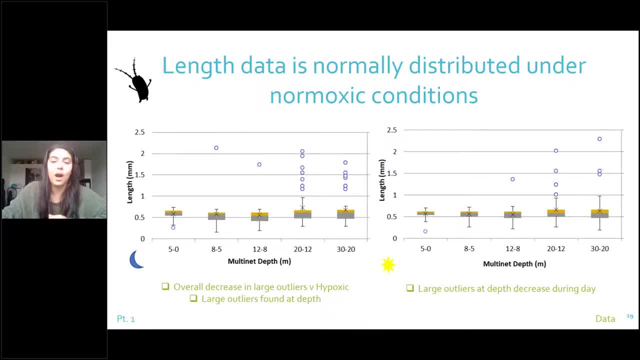 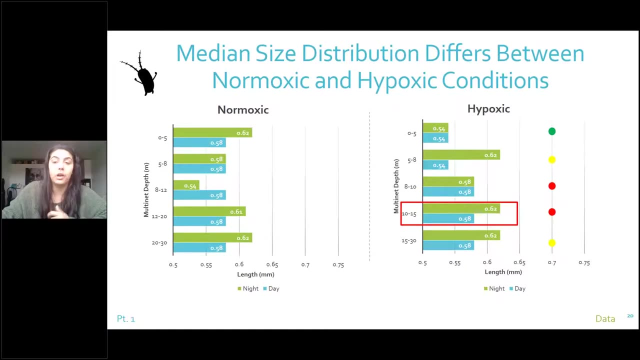 that was difficult here is the copepods have a very wide size distribution and there were a lot of outliers and considering outliers drew up the average value of length data in each depth strata. I switched to looking at the median to get a better picture of the copepod size distribution. 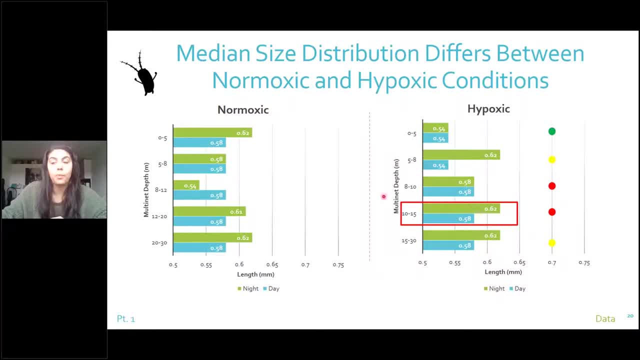 with the y-axis representing the copepod prosome length in millimeters and the x-axis wait, no, sorry. the y-axis is the multinet depth ranges and the x-axis is the copepod prosome. apologies Again. recalling my original hypothesis, this is where I expected to observe the smallest copepods at night. 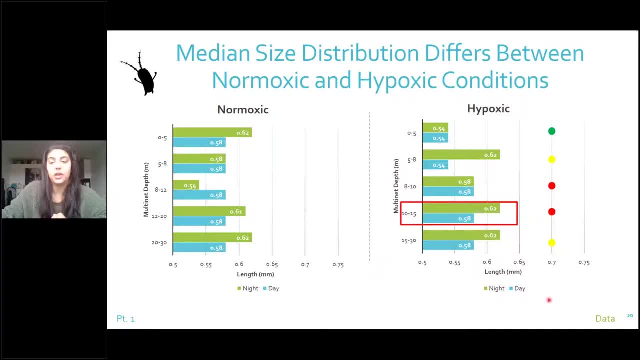 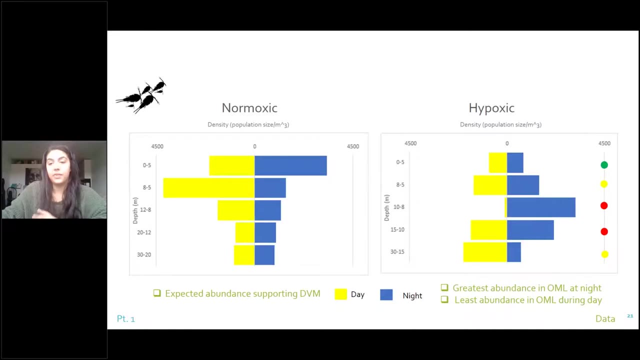 in the oxygen minimum zone, the 10 to 15 meter range under hypoxic conditions, and this data still did not support that hypothesis. Now moving on to my second question: how does oxygen affect the abundance of individuals? No, this is my abundance slide indicator. 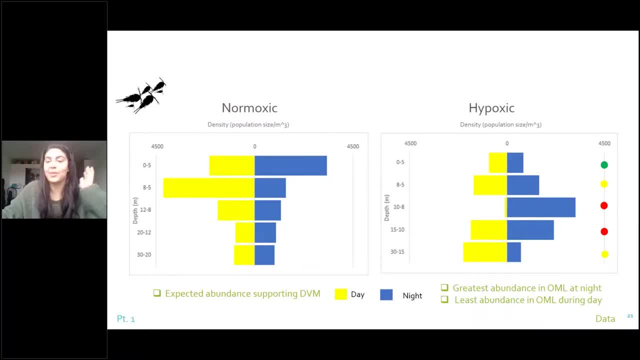 We're no longer talking about population density, we're talking about size. So temporarily forget about those graphs I just showed you. Regarding divertical migration, under norm moxa conditions we would expect to see copepods rise from the depths of the water column to the surface to feed, and that correlates to an. 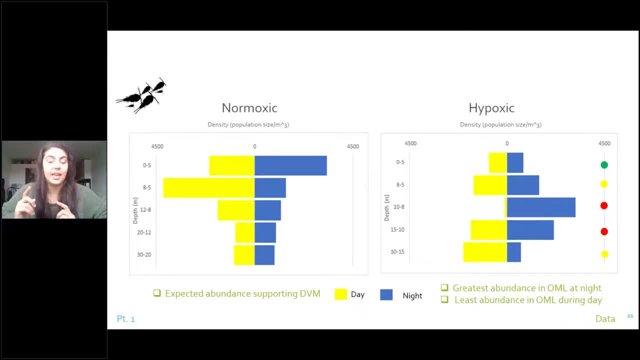 observed population density: highest in the surface waters at night, when light intensity has no influence on size distribution, and lowest during the day, as copepods migrate deeper and darker to the surface. Here we have two graphs of the estimated copepod abundance per cubic meter under normoxic and hypoxic conditions. 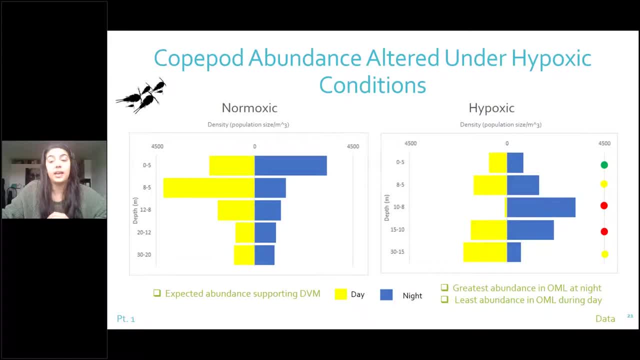 day represented as the yellow bars and at night represented as the blue bars. The y-axis represents the depth in meters and the x-axis represents the density determined as population size and density. The y-axis represents the depth in meters and the x-axis represents the density determined as population size and density. 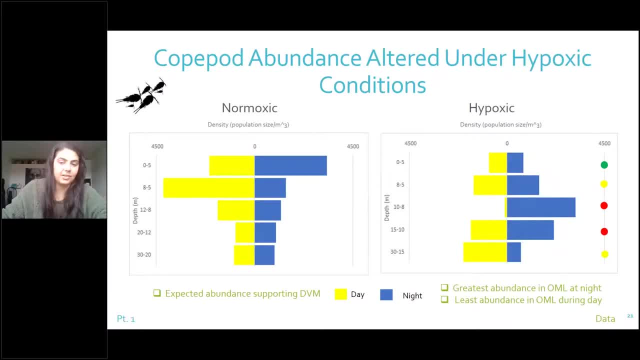 The y-axis represents the depth in meters and the x-axis represents the density determined as population size and density. Note the oxygen concentration indicators. my little, my dots. So again, right here in these two depth stratas we had severely hypoxic conditions and we just had hypoxic here. so that's a little. 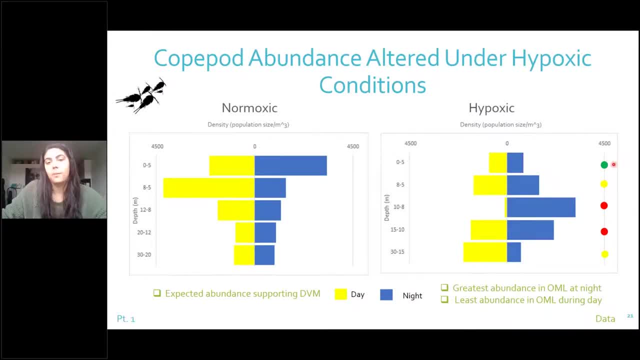 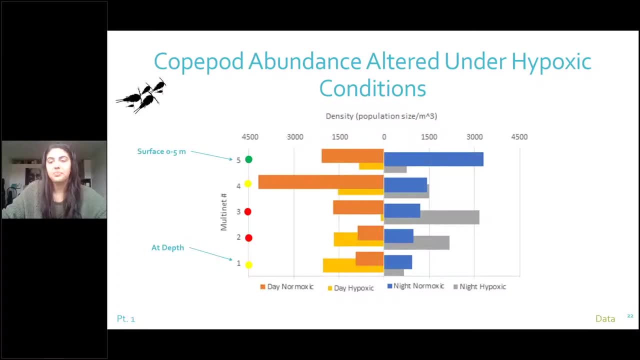 less than two milligram, two milligrams per liter and it was overall normal oxygen profile in a zero five meter range. we have a similar graph with normoxic. the orange and blue and the lower hypoxic yellow and gray conditions overlapped. to emphasize the difference, The y-axis depicts the multinet number with five. 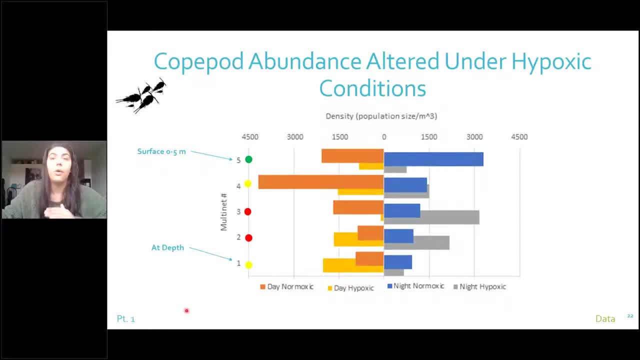 being at the surface and one being at depth. Now, remember, I'm shifting to multinet numbers because the depth ranges are custom to each oxygen profile. So because I'm looking at normoxic compared to hypoxic, the depth range is a little different. So I'm just going to show you the 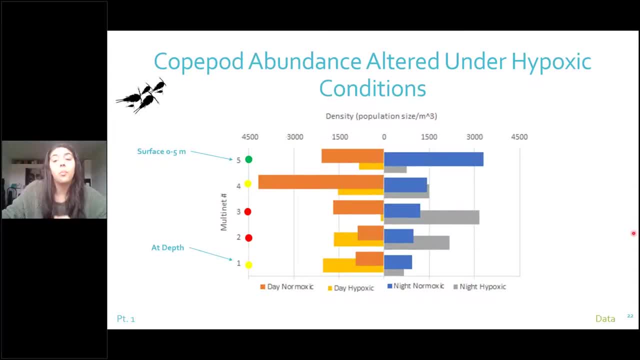 multinet range Under normoxic conditions- the orange and blue- we found evidence to support the theory of divertical migration, with the highest abundance in the surface zero to five meters at night and shifting down and in the water column as ambient light is introduced. 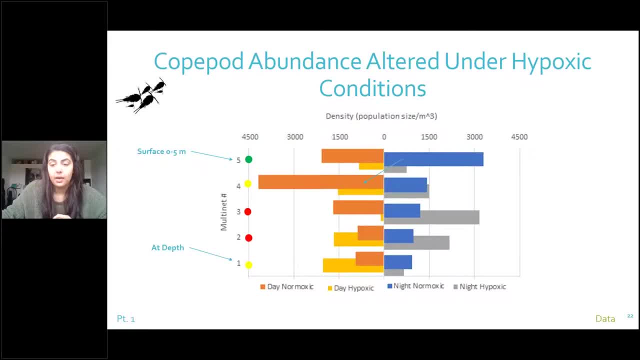 Under hypoxic conditions- the yellow and gray- we did not observe the traditional divertical migration behavior. Population density was actually highest in the hypoxic layers at night, So that's multinets three and two, and lowest during the day, meaning a large proportion of the population did not make it to the surface at 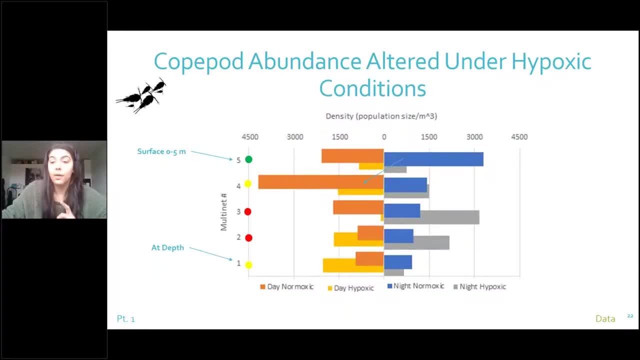 night under hypoxic conditions. This observed copepod abundance may support two previous studies theorizing that copepod abundance may support two previous studies theorizing that copepod abundance may support two previous studies theorizing that copepod abundance may exploit the oxygen minimum. may exploit the oxygen minimum as predation refuge. However, it's very curious why we 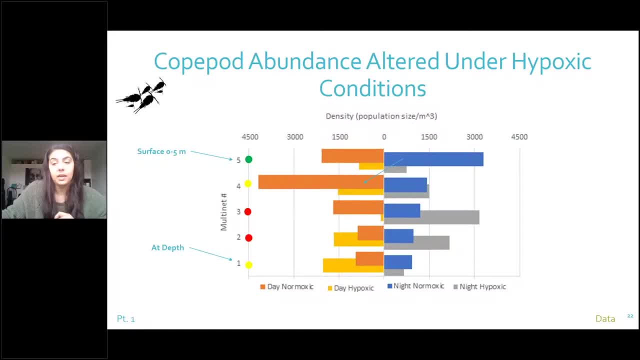 observed the dramatic shift in abundance from night to day, just above the oxygen minimum in multinet three. The hang up with our sampling method is we can't determine if the copepods are hanging out to avoid predation or if they're dead. So the null hypothesis. 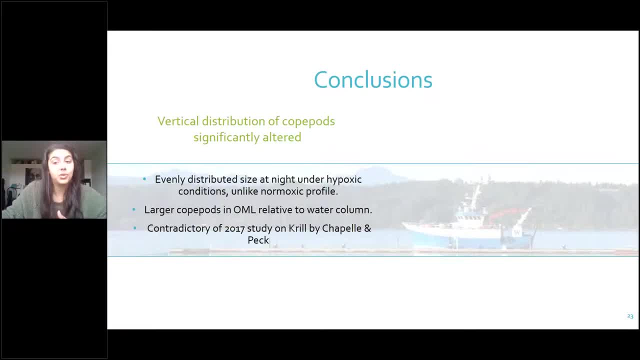 and relatively large copepods, occupying the oxygen minimum during both day and night, which is contradictory to a 2017 study on krill that observed the largest species and areas where oxygen concentrations were the highest. And regarding divertical migration, our abundance data support the theory of DVM. 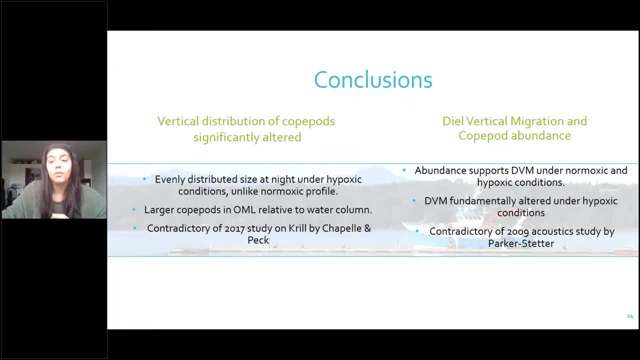 under both normoxic and hypoxic conditions. However, DVM was fundamentally altered under hypoxic conditions, which is contradictory of a 2009 study which concluded the oxygen minimum layer affected DVM but did not prevent it. My theory is under hypoxic conditions. copepods attempted DVM at night, but majority got caught in the oxygen minimum layer and either migrated back down to depth as ambient light was introduced or died and settled down the water column. If the vertical distribution of the size of copepods is significantly changed, this could affect predator. 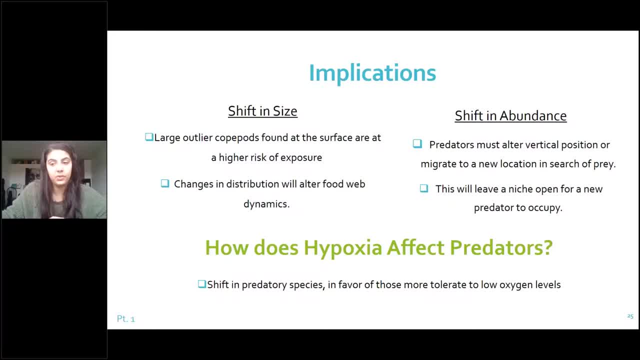 or prey interactions and alter the transfer of energy throughout the marine food web. We observed a shift in copepod size, with a more even distribution and size throughout the water column under hypoxic conditions relative to normoxic conditions. These larger copepods here at the higher surface levels 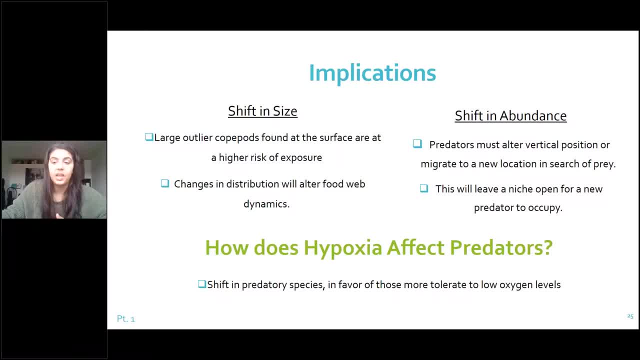 have a higher risk of being eaten by visual predators. If they're distributed differently, they can be exposed to different predators which will affect the, which will alter the food web dynamics. We also observed a decrease in abundance of copepods present in the surface layers under hypoxic conditions. due to either mortality rates or predator avoidance. It's unclear at this point. If predators do not adjust their position in the water column, they'll need to migrate to a new location in search of prey, leaving a niche open for a new predator to occupy. 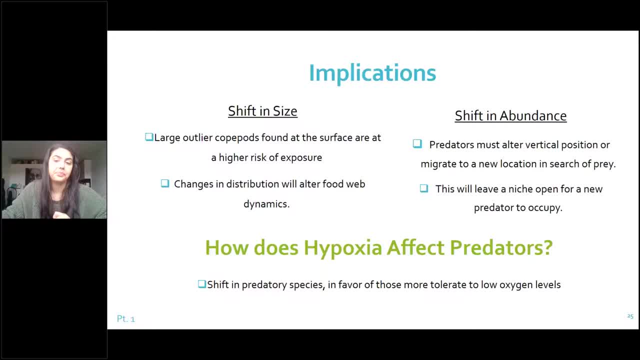 But what if predators are unable to adapt to low oxygen availability? This will lead to a shift in predatory species in favor of those more tolerant to low oxygen levels, who may have different predation behavior, like jellyfish or other gelatinous species. Since graduation, I've continued to work. 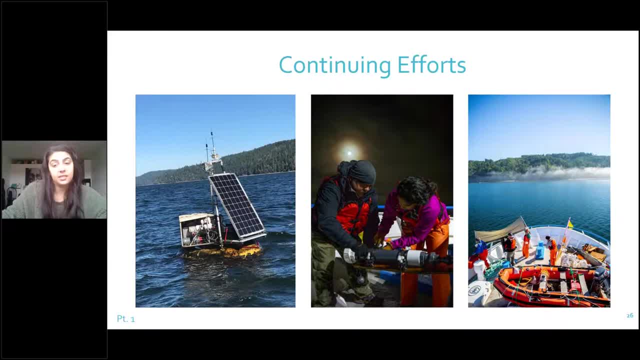 with doctors Keister and Grunbaum to develop an imaging system to observe zooplankton swimming behavior in situ, with the hopes to add more data to this study. Net tows are just snapshots in time, but with imaging we can look up and down the water column. 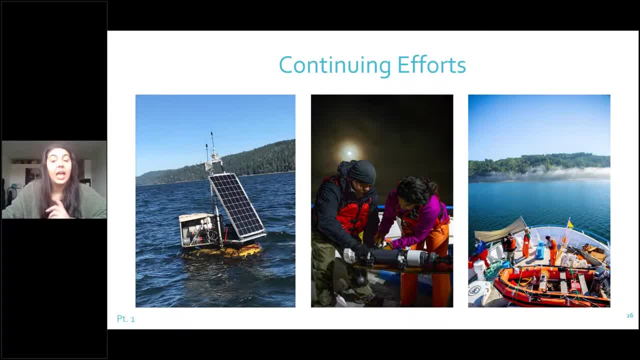 to get a better idea of what's happening beneath the surface, An imaging system was deployed on the Tawana Orca mooring from May through September from 2017 to 2018 to monitor zooplankton abundance, vertical distribution and small scale movement behaviors from prior 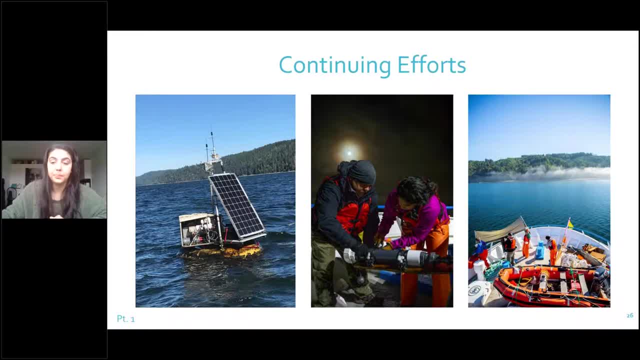 to the onset of hypoxia through peak hypoxic conditions. The system profiled the water column several times a day to resolve changes in distributions on dial to seasonal timescales. We also built and deployed an array of low cost video cameras on Lagrangian drifters. 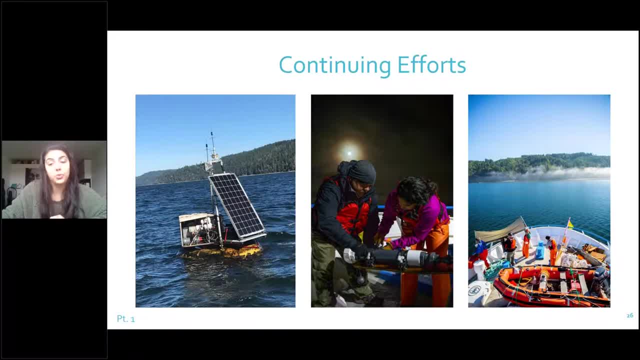 at four depths to concurrently study the behaviors and distributions of zooplankton throughout the water column and the hours surrounding sunrise each day. to capture zooplankton vertical migrations from surface to depth, when they're most likely to experience changes from favorable to unfavorable conditions. 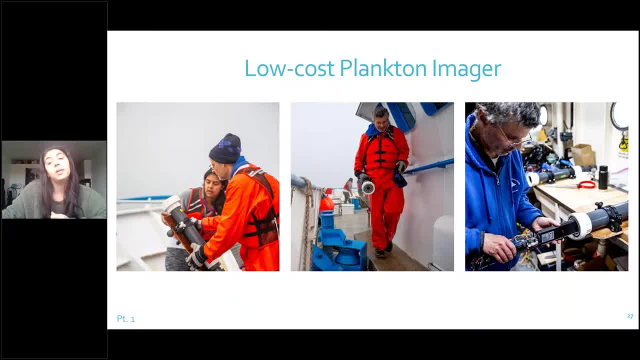 Dr Gruenbaum developed a low cost plankton imager to be mounted to the Lagrangian drifters, which included a camera and infrared illuminator and battery pack which was constructed using only off the shelf and 3D printed parts. 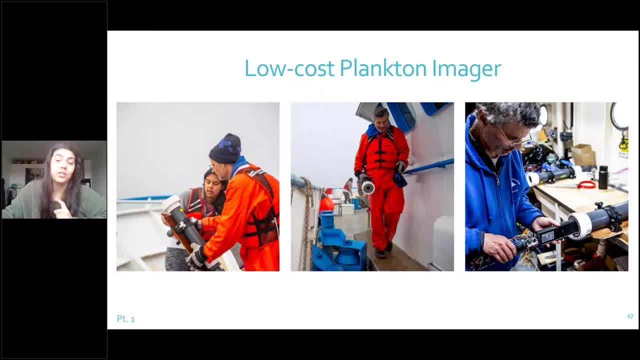 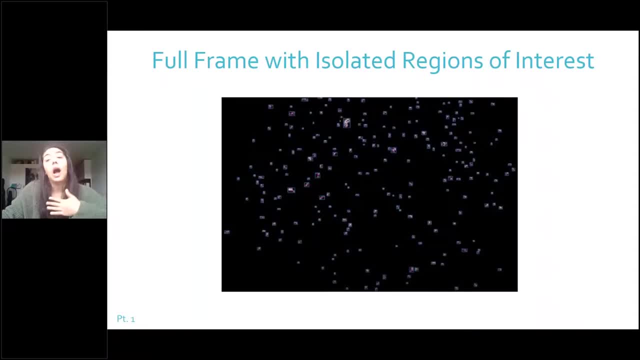 This imager can collect up to 60 gigabits of video during a 24 hour autonomous deployment. I personally work with an array of still images collected from the Orca moorings. Particles that fit a predetermined size threshold are identified and isolated for manual classification. 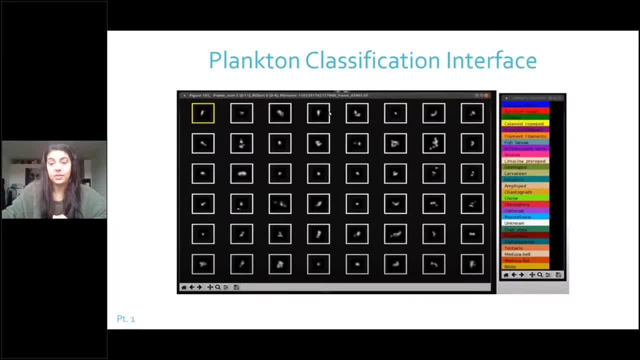 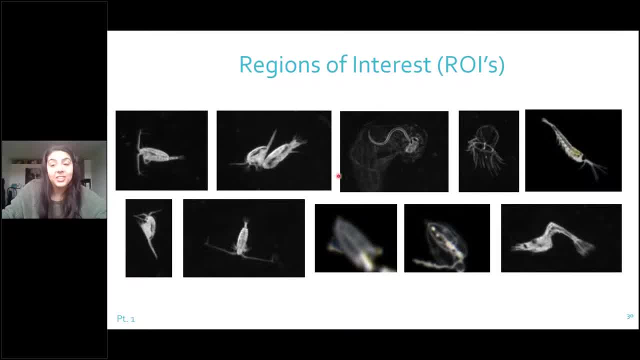 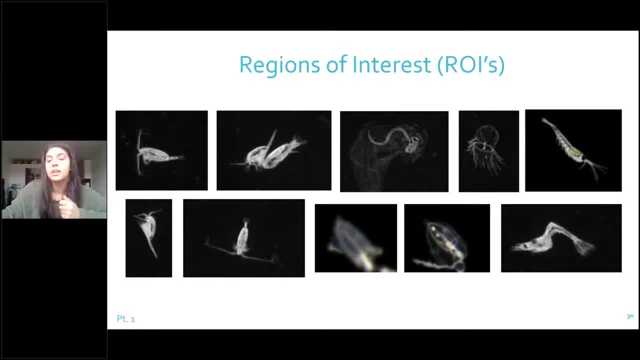 All of the classified ROIs have their own corresponding timestamps, depths and CTD profiles associated with them, So we're able to identify the specific conditions we're observing them under. It's truly some really exciting work, And I think that's what we're doing right now. 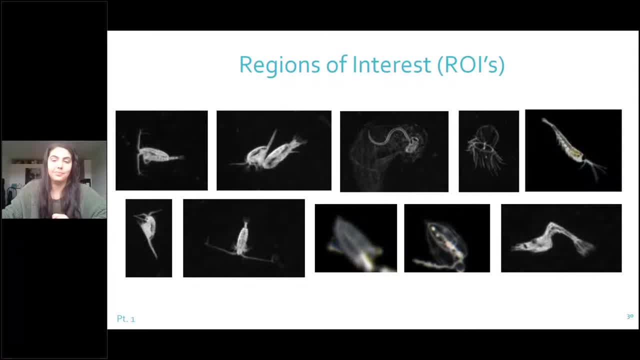 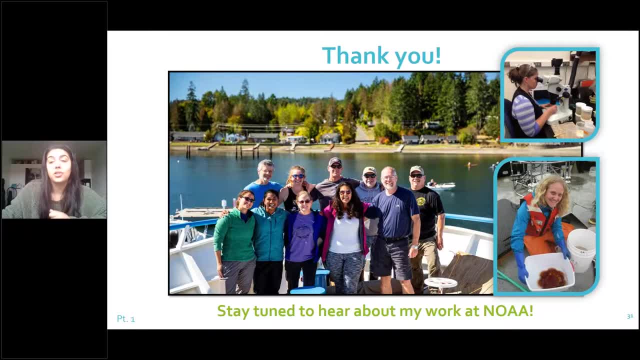 And getting beautiful images like these are the highlight of my job, The skills I gained working with Dr Julie Keister and Dr Danny Grumbom, their graduate students Sasha Soroy and Amy Wyatt, and the training I obtained from their research scientists. 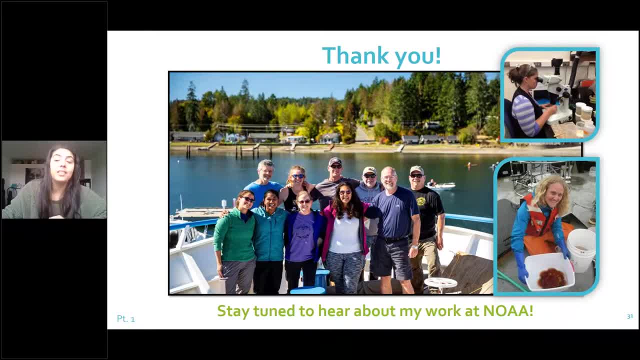 and technician Amanda Winans and Bethely Herman have made the transition to my work here at NOAA seamless, So I owe a big thank you to them, And I know a few of them have tuned in in support of me here today. so thank you, ladies. 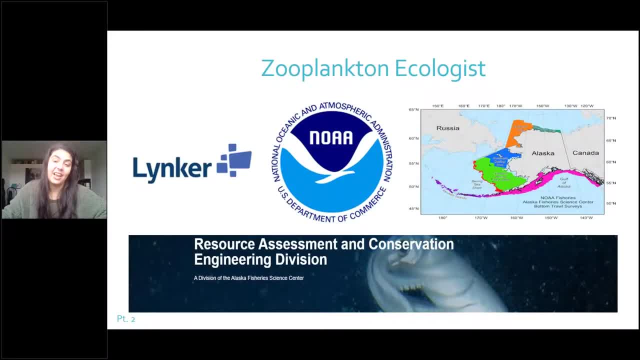 Now for the second portion of this presentation. I'll share my current work here at NOAA, where I've been given the opportunity to further my skills in taxonomy and image analysis. I'm actually a contractor with Linker at NOAA's Alaska Fishery Science Center and the Race Division here in Seattle. 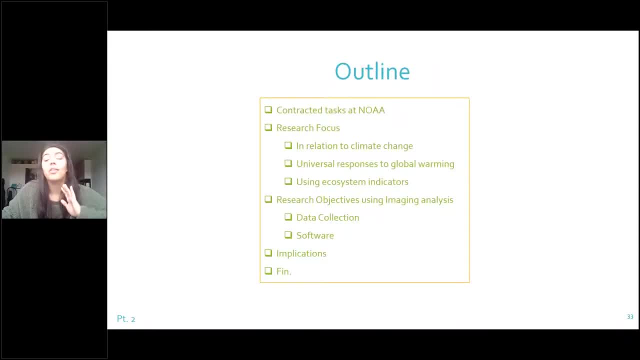 Now I'm going to cover a lot of topics and jump around a bit, So here's an outline, so you know what to expect. I'll go over my contracted tasks at NOAA, then I'll shift into my research focuses, which are in relation to climate change, universal responses to global warming and using ecosystem. 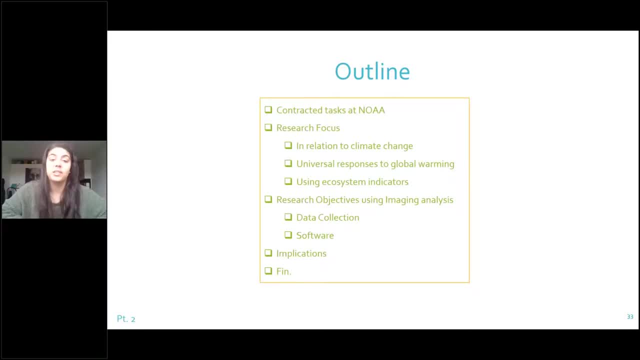 indicators. Then I'll go over research objectives using imaging analysis, from my data collection to the software we're going to use, as well as implications of our findings for this overall health of our ecosystems. All right, so here we go. A large portion of my work here consists of zooplankton identification. 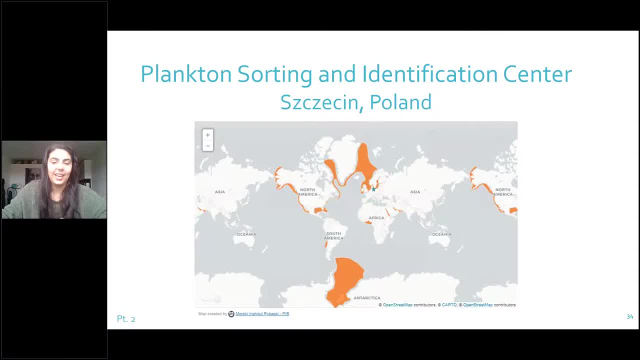 NOAA has been in collaboration with the Plankton Sorting and Identification Center, located in Szczecin, Poland, for 45 years. The department was founded in 1974. Following the census, It was established in the 1970s following the signing of an intergovernmental agreement. 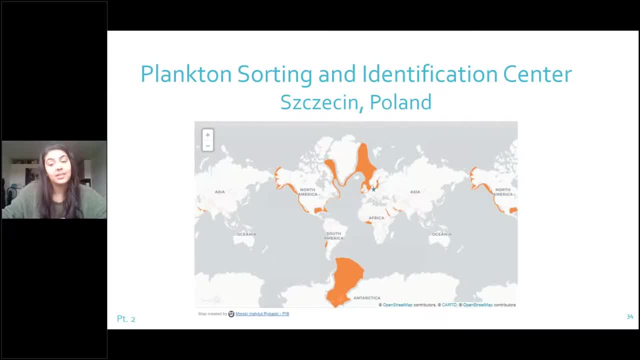 between the Sea Fisheries Institute in Gdynia, Poland, and the National Marine Fisheries Service in Woods Hall, USA. This creation of this sorting center was actually stimulated by a 50% decrease of bottom and pelagic fish resource biomass in the Northeast Atlantic in the 70s. 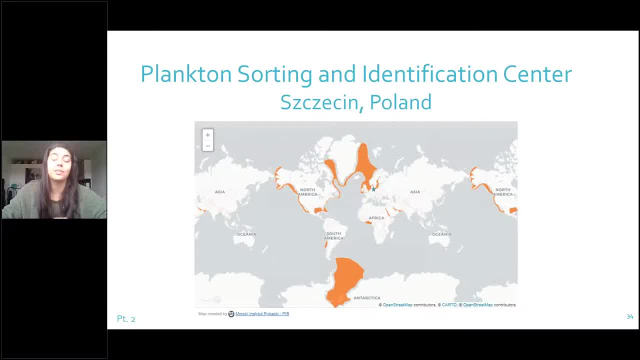 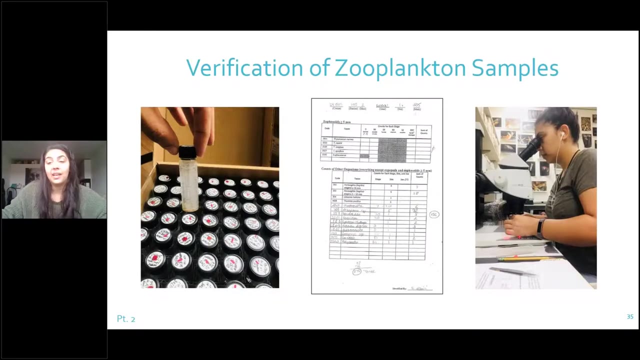 Currently there are about 10 highly skilled women that work here who process over 7,000 zooplankton samples a year from all over the world. So you can see, the orange is all the different oceans that they process. samples from All of the zooplankton samples we collect here at ASFC are shipped to Poland, where 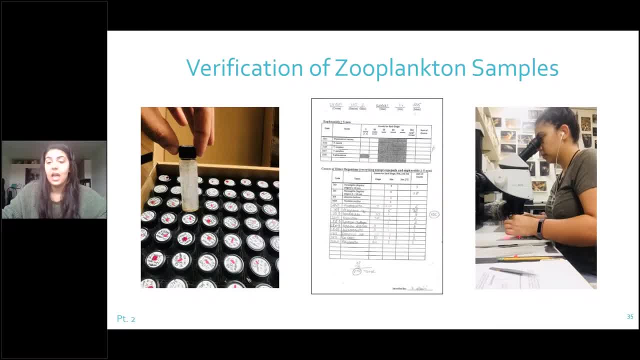 every specimen is identified, sorted and recorded, And then they're shipped back here to Seattle, where Jesse Lim and I QAQC this data through a verification process. The samples are then stored in our archive room, Where we have records of specimens dating all the way back to the late 80s. 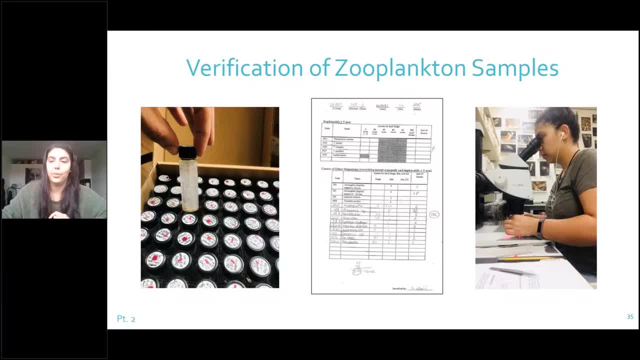 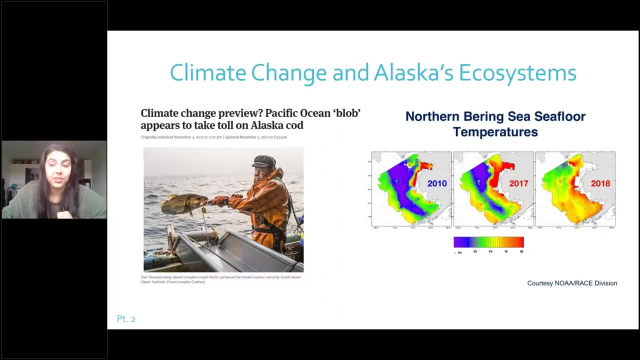 So this is what my normal day-to-day work looks like here at NOAA. Now I'm going to shift to my research and what I'm really interested in, which is looking at climate change in Alaska's ecosystems. The marine ecosystem off Alaska's coast sustained North America's richest fisheries. 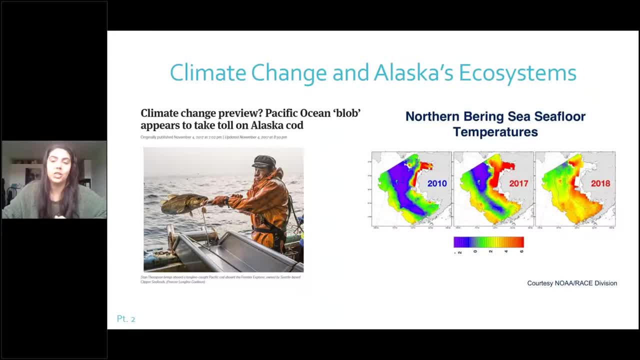 Alaska exports more than 1 million metric tons of seafood each year, bringing in over $3 billion worth of new money into the US economy. Warming ocean temperatures, which peaked in 2015,, are believed to have had a major effect on the health of our fisheries. 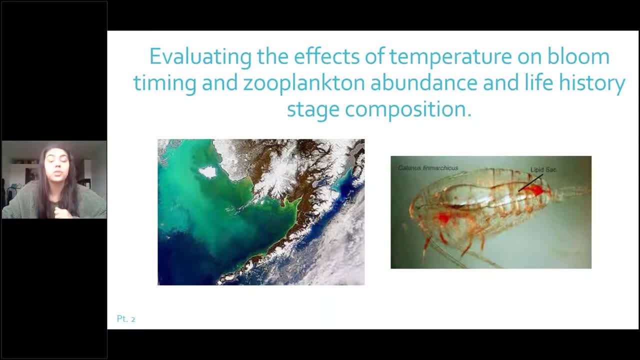 Now there are many things that can affect plankton growth, which is really important to our ecosystems because it sets up the base of the lower food web. One of the effects of warming waters is we're beginning to see an early sea ice retreat on the eastern Bering sea shelf. 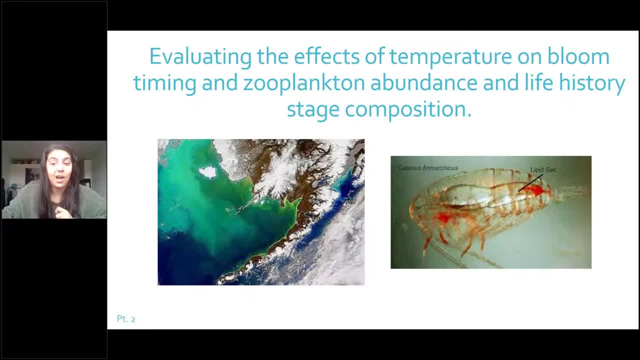 And this early sea ice retreat is triggering an early spring algal bloom. Now, zooplankton vary their activities and reproduction according to the season And we believe the timing of the spring bloom is critical to them. It's when and how they get the nutrition they need for egg production. 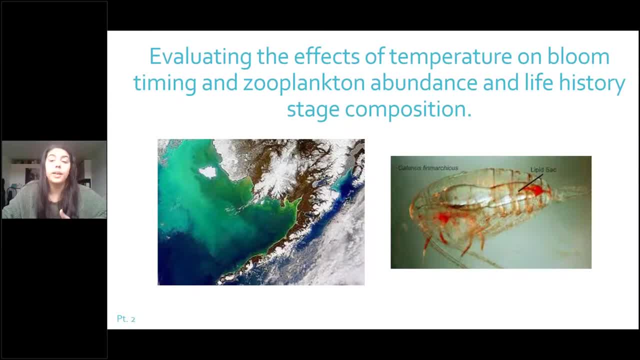 The mismatch of when food is available and when zooplankton come out of diapause and search for that food could send ripples up the food chain. So this is just one of the things that I'm currently looking at, but I'm not going to. 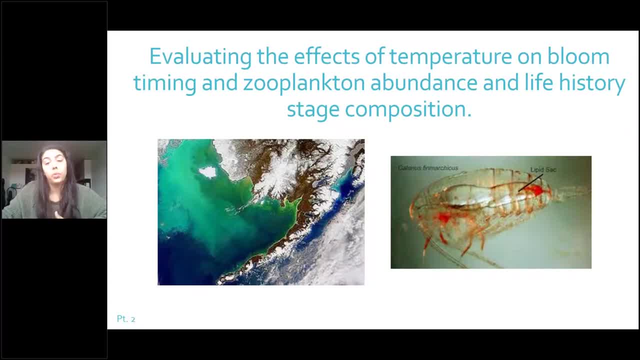 talk more about this today. Instead, I'm going to focus on zooplankton and how they serve as an important link to the overall health of our ecosystems- One of the many things that I'm really interested in. One of the many things that I'm really interested in. 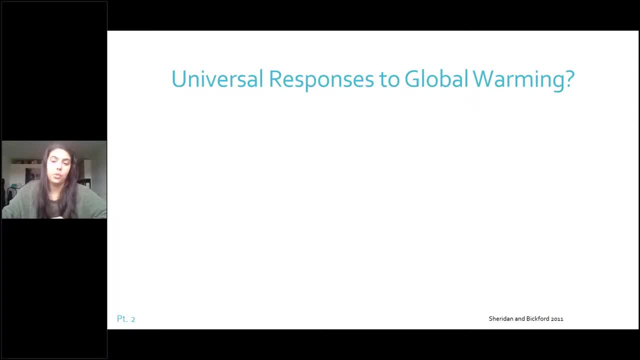 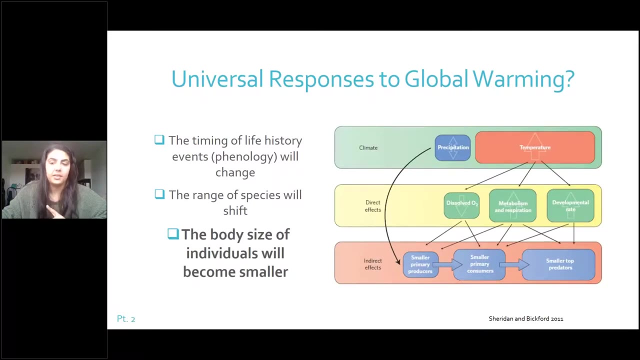 Are the universal responses to global warming. Now, the first two bullet points are pretty well documented. that will see responses to phenology and range species shifts. But this third one is still hypothesized, with only some evidence to support it And when you consider the effects of a small zooplankton body size across ecosystems. 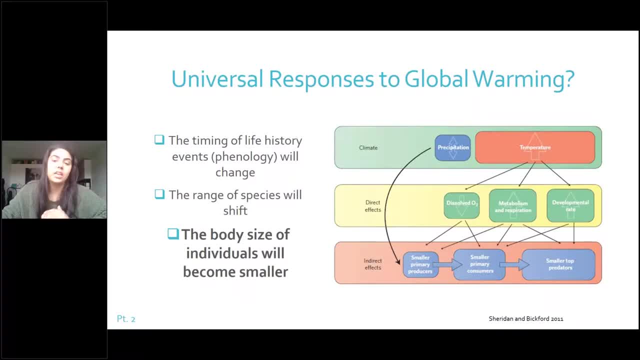 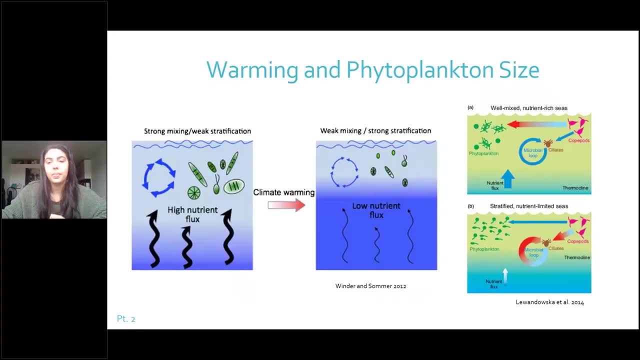 there is even less evidence at hand. So it's really an interesting topic to focus on for our seas that we monitor here at AFSC. So it's really an interesting topic to focus on for our seas that we monitor here at AFSC. We researched some well mixed, nutrient rich seas, and an example of this is the Bering. 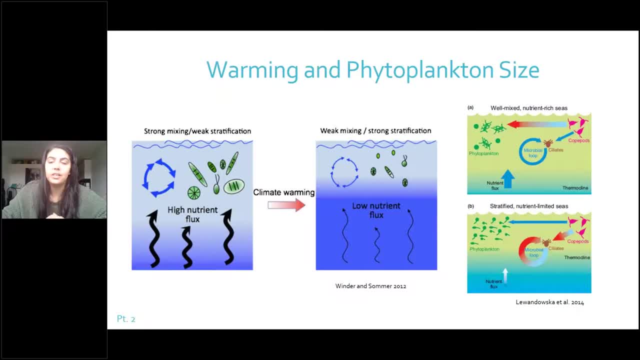 sea shelf, which tends to have this period of really strong mixing. When you get phytoplankton blooms and then it stratifies, You'll see a division in the water column into layers with different densities, which inhibits nutrient flux. Now, if we begin to see an extension in the length of stratification or how long it lasts, 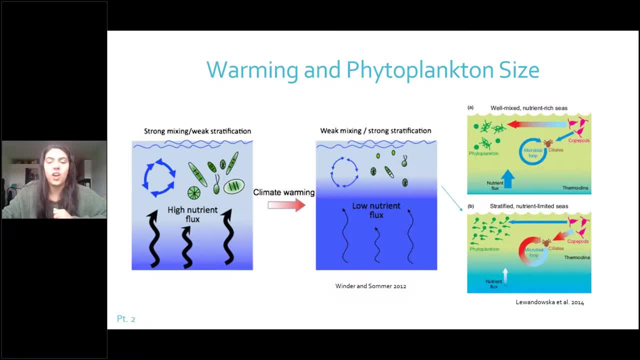 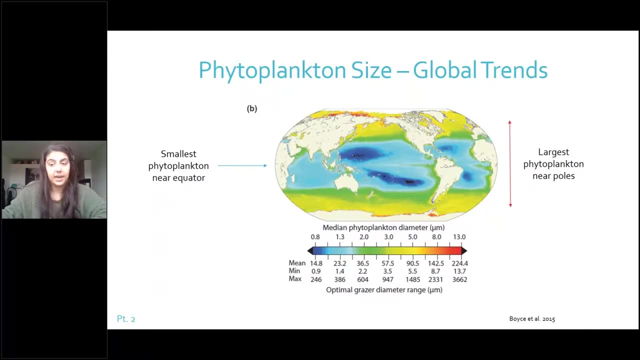 then we're going to see a shift toward this more stratified, nutrient limited situation, which, in turn, will affect the food web in terms of overall carbon and energy flow. Looking at global trends and phytoplankton size, We can see the smallest phytoplankton. 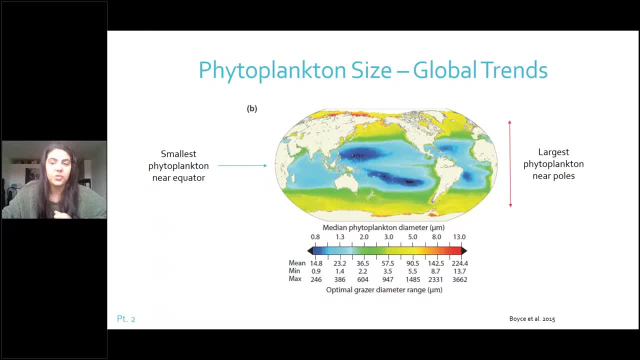 We can see the smallest phytoplankton are observed near the equator, where sea surface temperatures are warmer and increasing in size as we move towards the poles and temperature decreases. This is where we expect to observe highly productive ecosystems, at the poles, in the 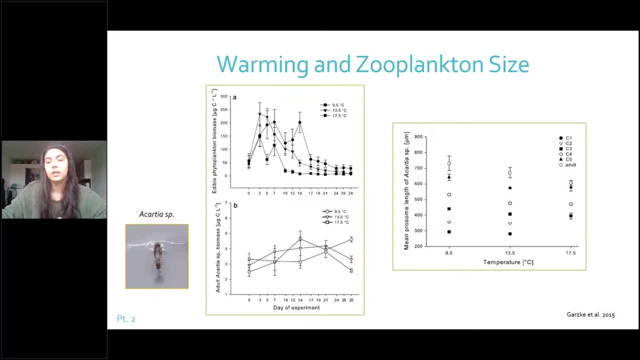 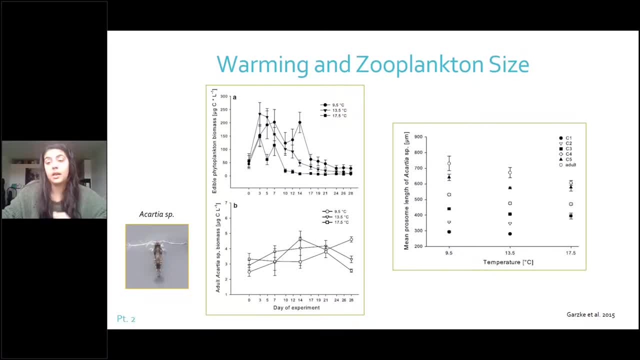 conditions by performing a mesocosm experience experiment using plankton from the Baltic Sea at three temperature levels, So 9.5, 13.5 and 17.5 degrees Celsius. Look at the average biomass of edible plankton phytoplankton. there's an overall decrease. 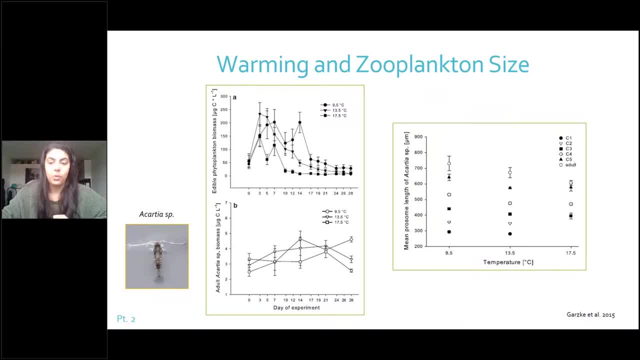 in the lek quintet around 1.2 to 9.5 to 19.5 degrees Celsius per unit At 6,, 16,, 17,, 58.. There's truly no standards for this measurement over time: 13,, 16,, 17,, 88.. 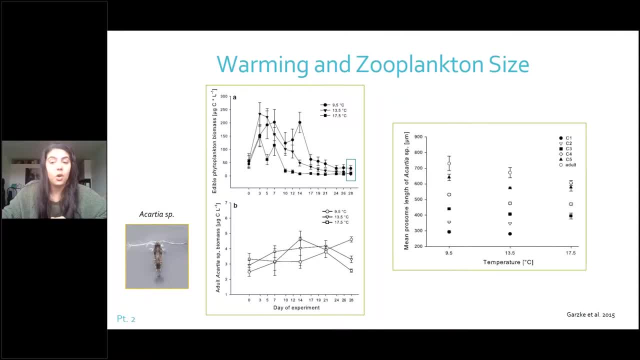 CAGR 36, ah, caenowa segrecia 36,, 6,, 61,, 74,, 48.. So for the average biomass of edible, plankton, phytoplankton in the biomass, regardless of temperature. 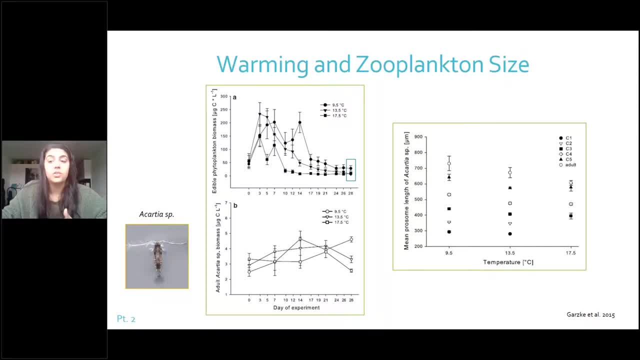 So we know over time, in a mesocosm, zooplankton are grazing on phytoplankton. Now, looking at the average biomass of adult acartia, a species of copepod, over time we see the coldest temperatures, the open circles. 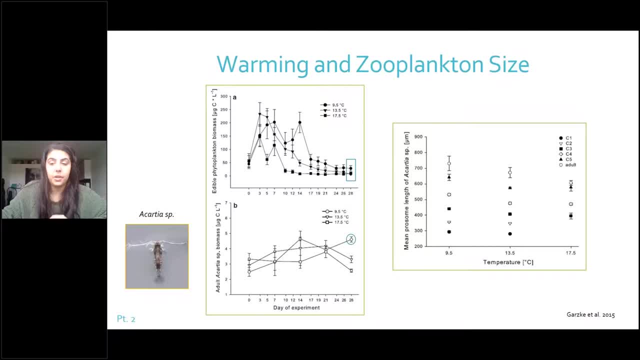 they have the most biomass, but in the warmest temperature- the boxes- they have the smallest biomass. So acartia growing under cold conditions are eating the same amount of food in relation to those growing under warming conditions, but they're bigger. 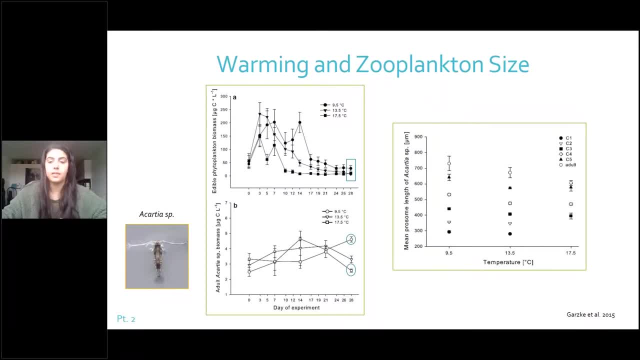 There's more biomass- roughly 50% more biomass. Now, again, this is just biomass, So to confirm they actually are getting smaller. we'll look at this third graph that describes the average prozone length, the length of the body excluding the tail. 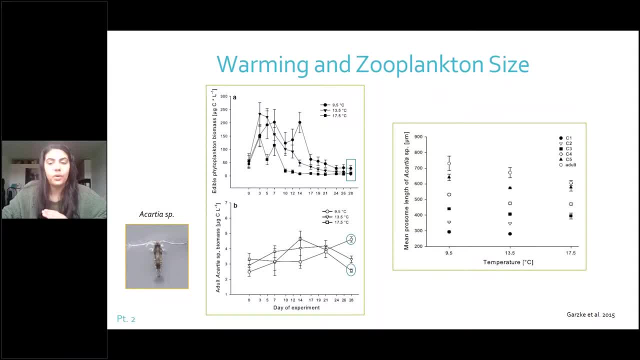 Looking at the 9.5 degrees Celsius and 13.5 degrees Celsius, we can see that the adults, these unfilled circles, are the largest. But when we look at the warmer temperatures- 17.5 degrees Celsius- we can see their prozone length is down about 100 microns. 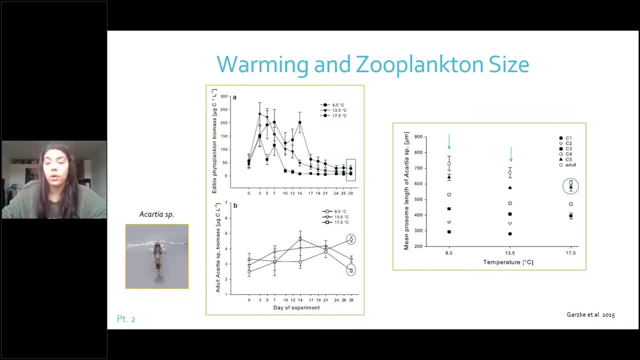 So they become more compressed as temperatures warm And it also gets less easy to distinguish between the C5, the filled triangles and the adult stage. The warmth is reducing their size. Their higher metabolic rates are inhibiting their ability to accumulate biomass. 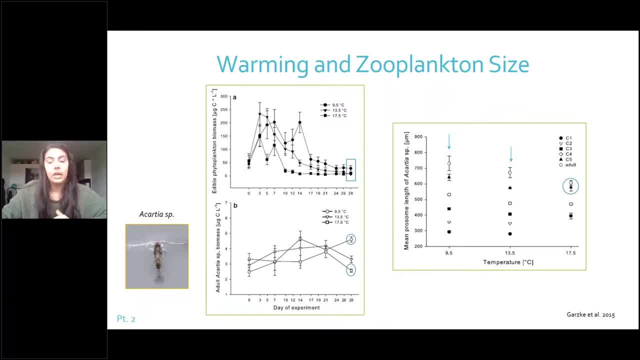 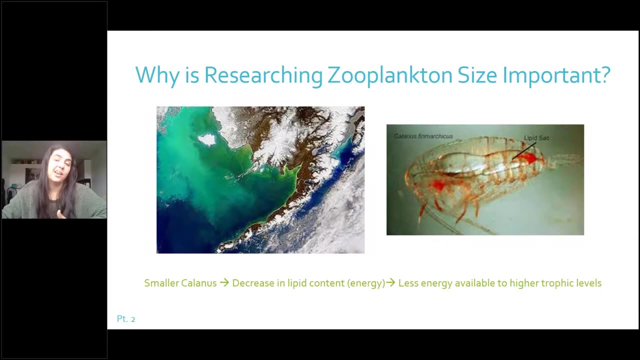 So this is what happened in a mesocosm. Based on this, what's going to happen in the Bering Sea with calanus, another species of copepod? If we extrapolate that data out to the Bering Sea, the individual cell size of phytoplankton may be smaller. 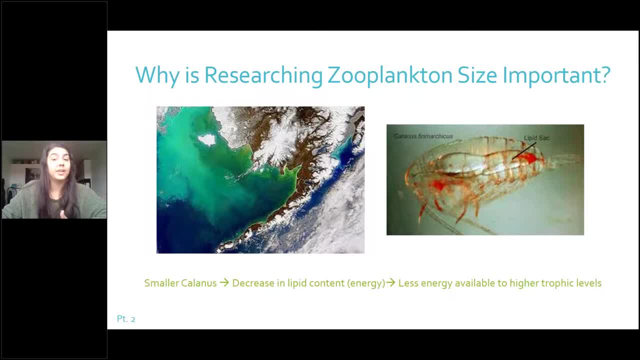 but overall there may not be major changes in relation to phytoplankton biomass. But if it gets warmer, we're going to have a population of calanus that are typically rich in lipid content, decrease in size And what we expect to see is size decreases. 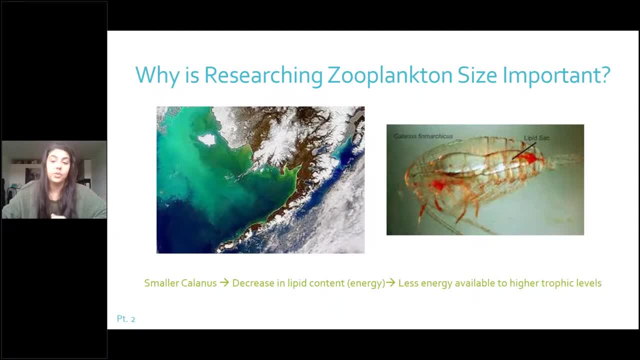 is, the amount of lipid, which is energy in the system, could go down and the size of the individuals could go down as well. So this is the lipid sac inside of a calanus. It's this little blob. it's kind of hard to see. 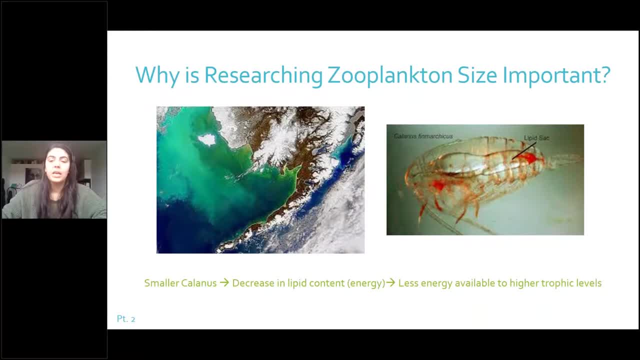 but it's like a little water drop. If the size of the individuals go down, this is going to affect how much energy is available to higher trophic levels. So how can we get some indications of whether or not this is happening? Are they getting smaller? 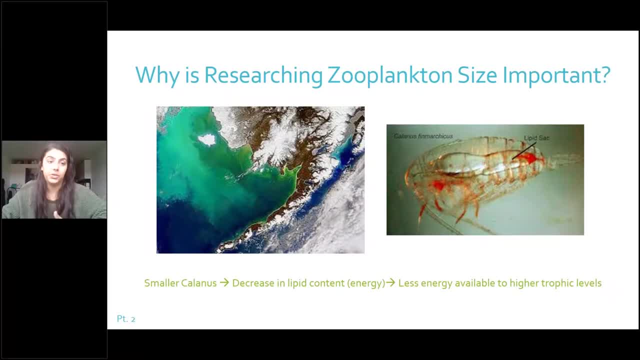 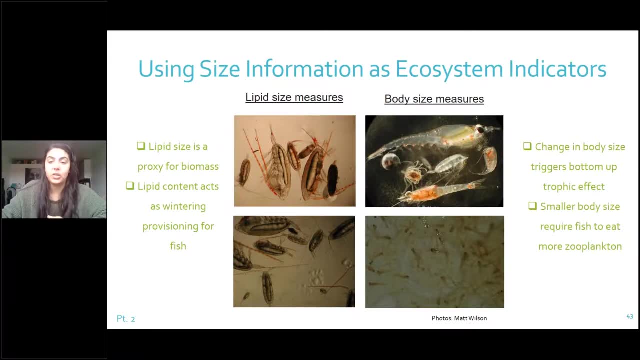 Are they less full of fat with less biomass? And how can we measure that? As it turns out, there is information that we can extract using specific size indicators. One is looking at the lipid sac and looking at the lipid size. So again here, these are the little. 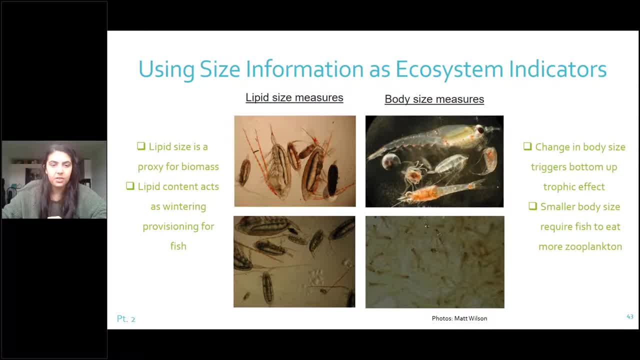 this is the lipid sac. We've got one right here, right here. They're a little hard to see, but once you get it you can point them out And we can use the lipid size as a proxy for biomass, because even if copepods are the same size. 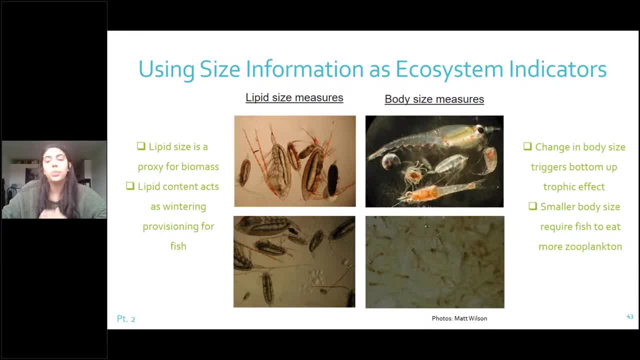 the amount of lipid content may vary, And lipid content is really important because it supplies overwintering provisioning for fish. We also have the ability to look at body sizes. If there's a change in body size measurements, we will observe a bottom up trophic effect. 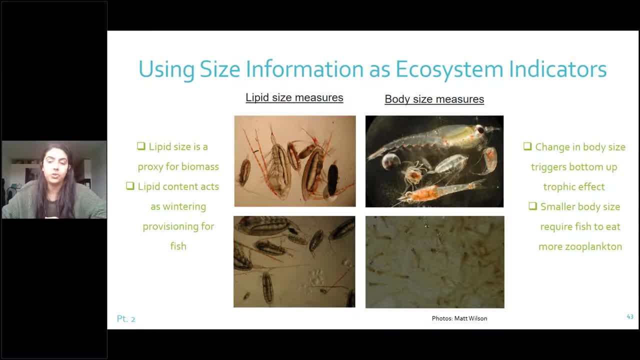 And fish will need to eat more zooplankton to get the same amount of nutrients as they did in the past. With image software, we can actually measure both of these things: the size of the lipid droplet and the body size Right. 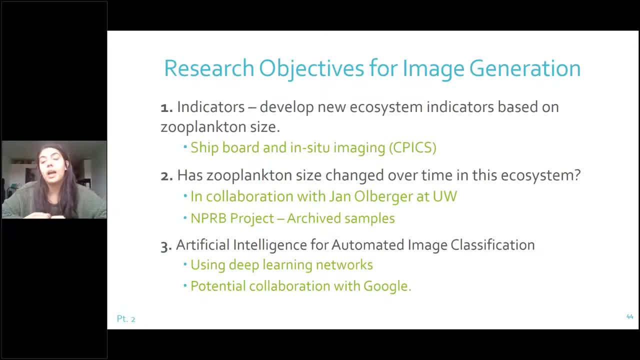 I'm now going to discuss my research objectives, which rely upon utilizing imaging analysis to identify trends in zooplankton size over time in Alaska's ecosystems. Keep in mind I'm just getting started with this research, So this is just going to be a general overview. 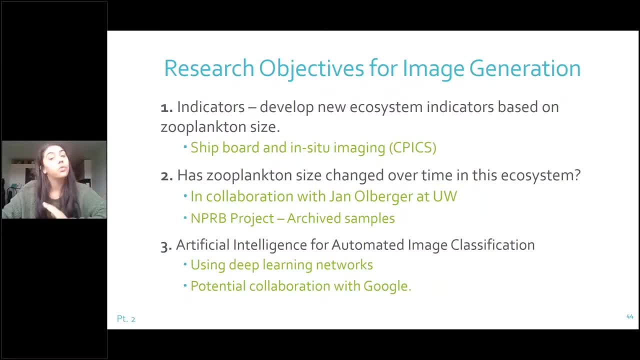 and some early shots of what we're working on. First, we're working on the development of new ecosystem indicators based on zooplankton size. We'll generate images using shipboard as well as in situ imaging. Next, in collaboration with Jen Ohlberger, 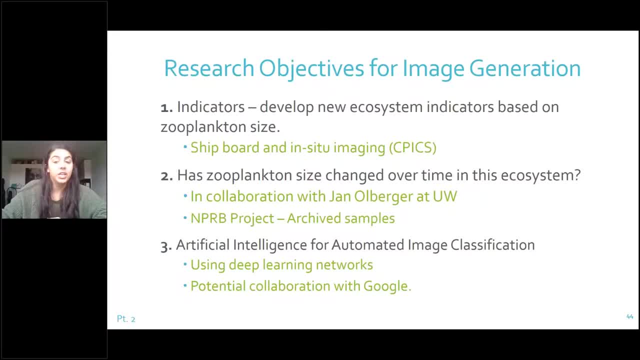 our goal is to determine if zooplankton size has changed over time, And we'll do this by utilizing our archive samples that we have here on campus. And the most exciting is, we're hoping to develop artificial algorithms to identify species automatically using a variety of deep learning networks. 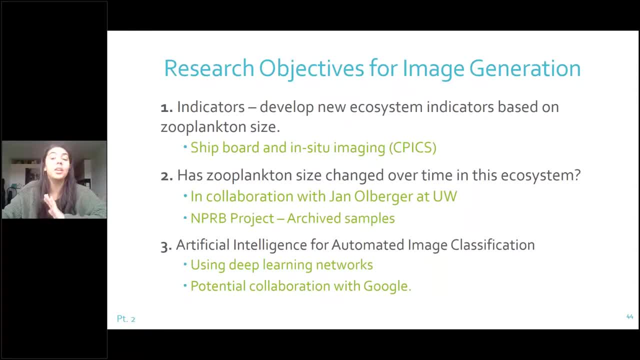 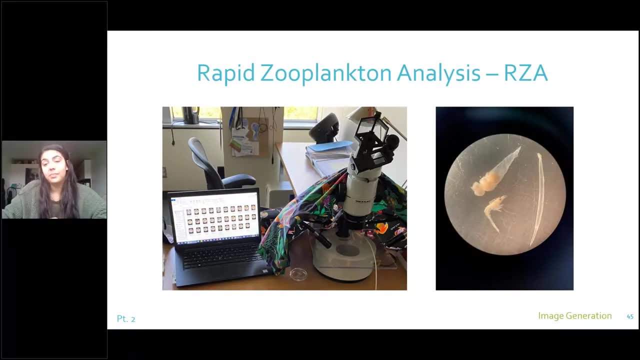 and a potential collaboration with Google. Now I'm going to show you how we're going to do this. In 2015,, AFSC implemented a new research tool called AFSC and method for an at-sea rapid zooplankton assessment- RZA. 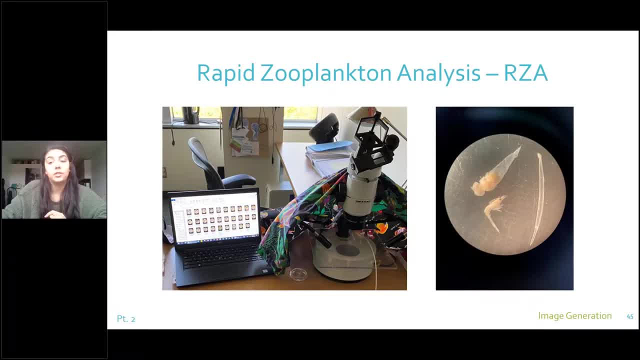 to provide leading indicator information on zooplankton composition in Alaska's large marine ecosystems. It was developed in order to provide information for our ecosystem status reports that I'm sure many of you are familiar with. This rapid assessment is a quick sort and identification. 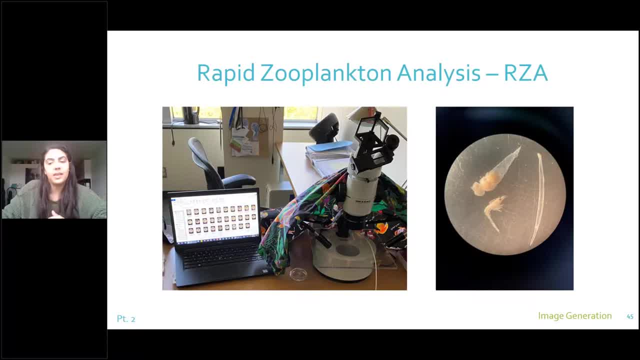 of the zooplankton community and provides preliminary estimates of zooplankton abundance and community structure. Through RZA, we'll be able to generate a number of images just using a simple microscope cell phone adapter, And with these images collected at sea. 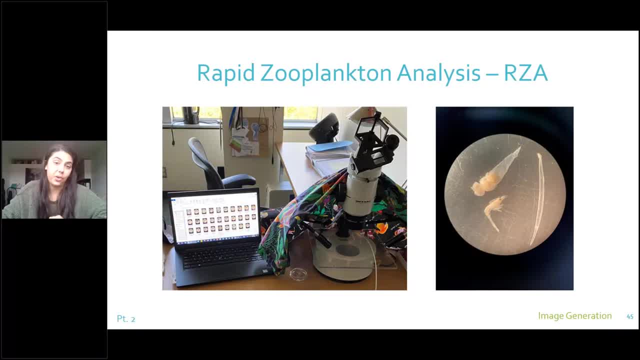 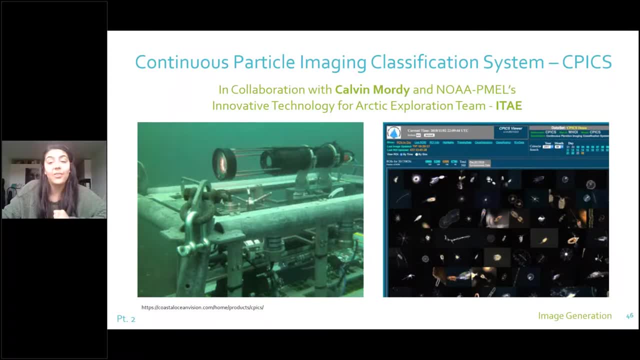 we can analyze and extrapolate size data using imaging software. We're also working in collaboration with Calvin Morty and NOAA PMEL's Innovative Technology for Arctic Exploration team To use this really, really cool continuous particle imaging classification system, which features embedded processing. 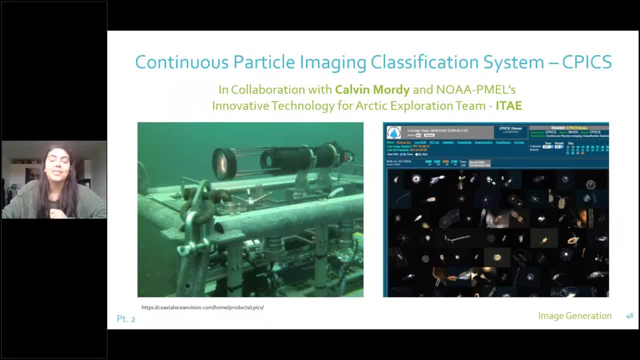 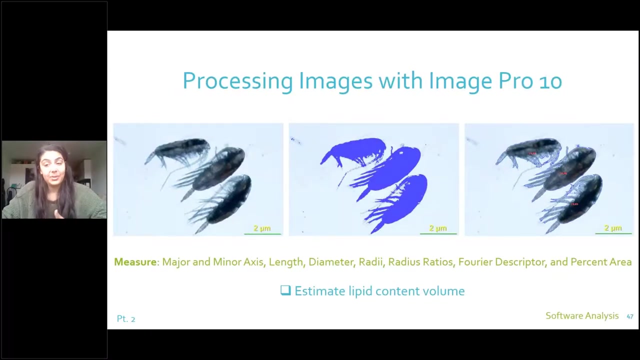 and region of interest extraction. it's capable of standalone deployment on CTD rosettes as well as via autonomous platforms or vehicles. This camera system is already trained in biodiversity of plankton and can automatically classify 22 species using deep learning, Once we've collected images at sea and in situ. 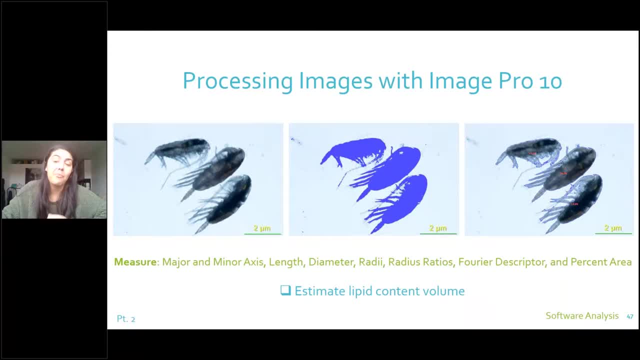 we can use the ImagePro10 software to batch, process and extrapolate a wide variety of size descriptors, as well as estimate lipid content volume. This software has the ability to identify regions of interest using a color contrast threshold, as well as the option to classify objects. 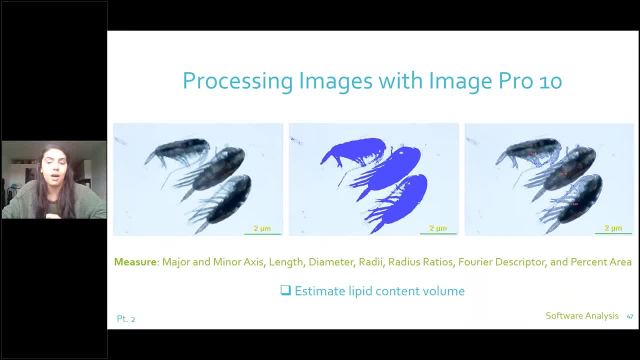 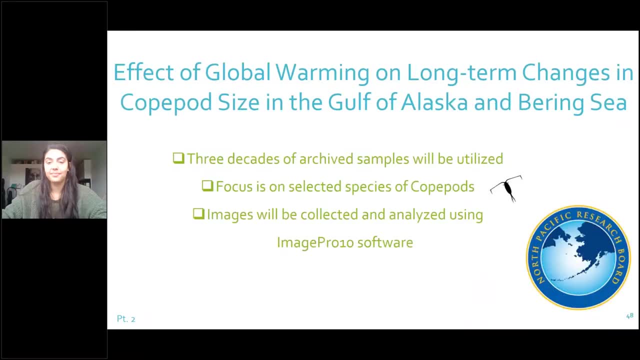 in order to train the program to become automated. once a large library is created, The large library of images are loaded into the system. We've also recently received funding through the NPRB to research the effects of warming on copepod size in the Gulf of Alaska and Bering Sea. 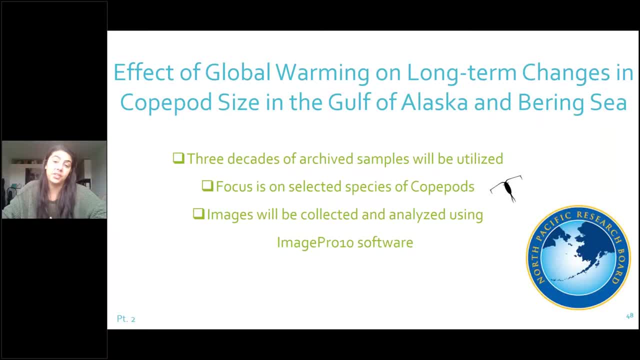 Both areas support important commercial and subsidence fisheries. We'll utilize three decades of archived samples to generate images of selected species in the Gulf of Alaska and Bering Sea, And we'll be using the ImagePro software I just showed you to analyze these images in order to quantify the effects. 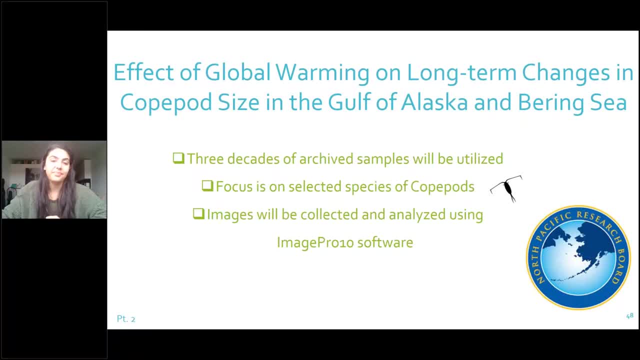 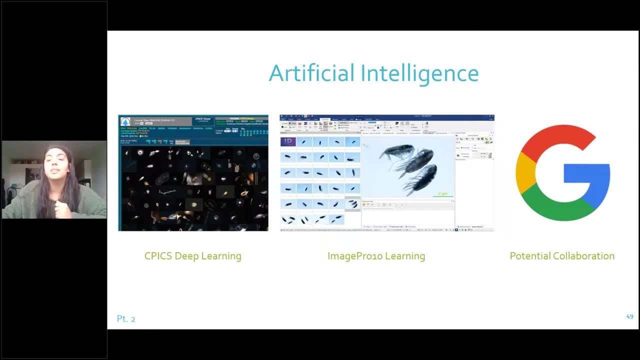 of long-term warming on copepod sizes. And finally, as I mentioned, we're hoping to develop artificial algorithms. We'll be able to take all of these images generated via the RZA, CPICS, the NPRB project, as well as a vast collection of images. 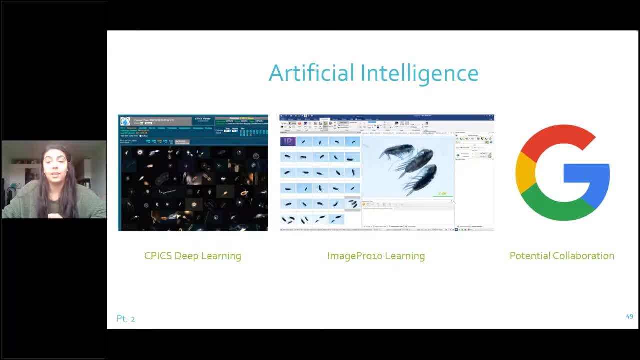 that are being generated in Poland in lieu of samples, we were unable to collect this year and begin classifying them in order to identify species automatically, using a variety of deep learning networks and potential collaboration with Google, which is really exciting and may also put me out of a job. 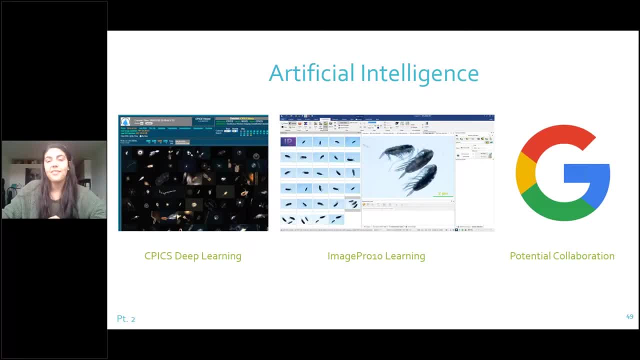 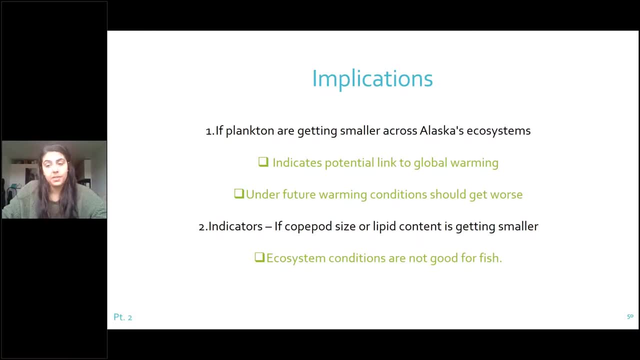 but I think that's a way down the way. This imaging work is just getting started, but if our hypotheses are confirmed and plankton are getting smaller across Alaska's ecosystems, it'll mean there's less biomass and lipid content available to fish and indicates a potential link to global warming. 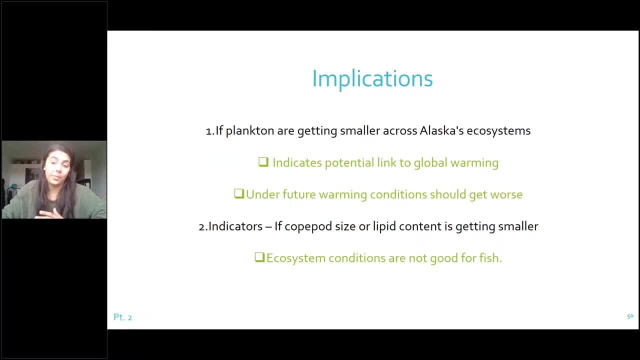 And if we know that, we'll know that under future warming conditions the decrease in zooplankton size will only continue and get worse, And if our developed ecosystem indicators confirm our copepod size or lipid content is in decline, implications for our ecosystem conditions that giving year 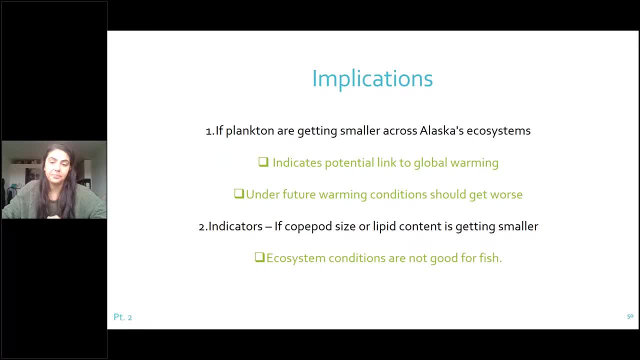 are not good for fish and, in turn, not good for our fisheries. Well, I hope over the past 38 minutes I've been able to convince you about how important zooplankton are. As I mentioned, this work is just getting started. 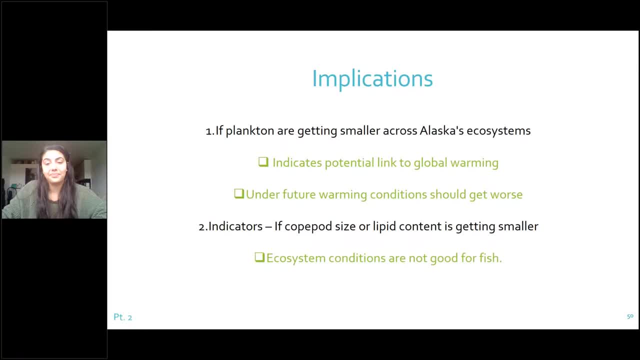 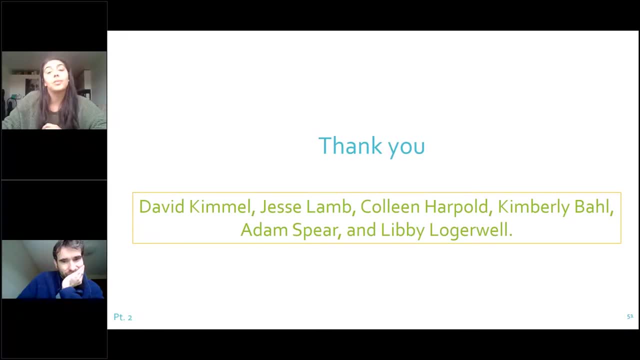 but I truly look forward to sharing my findings with you in the future. I want to give a special acknowledgments to Dave Kimmel, Jesse Lam, Colleen Harpold Kimberly Ball, Adam Spear and Libby Lagerwell for my help training me. 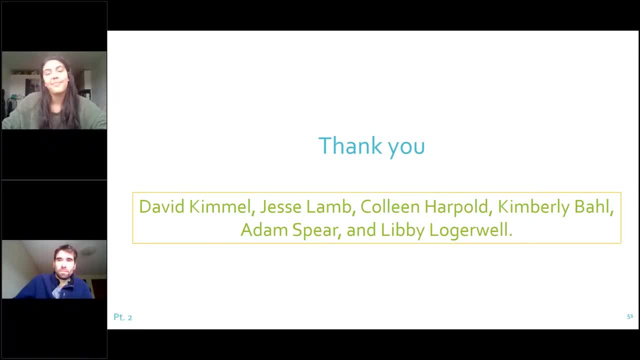 and getting me set up here at NOAA and helping me with this presentation. Thank you so much, Diana. You'll get the round of applause that Heather usually does. We have time for questions, So please, if you have all the 110, or I guess there are 90,. 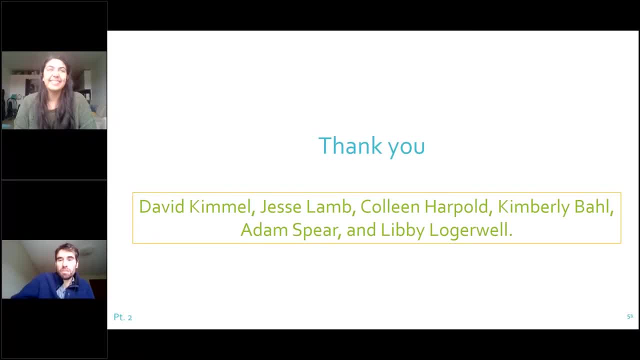 99 left huge crowd. if anybody has questions, please put them in the chat box. We'll start with one from Ned Coquelet, who is asking about your Toronto work. I'm just wondering. he says how deeply the light penetrated during the day. 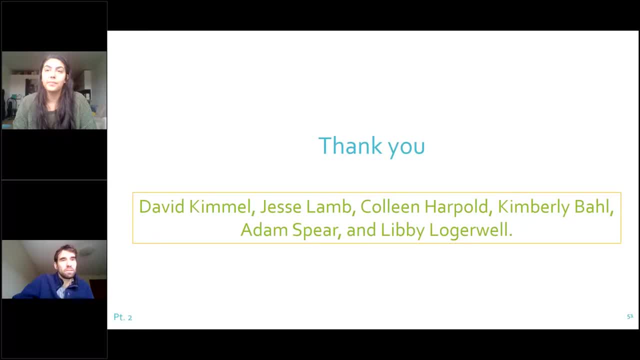 and its relationship to the depths of your plankton toes. Well, the graphs and profiles were mostly just looking at the oxygen concentration, so I didn't spend time, you know, looking at the oxygen concentration, so I didn't spend time, you know. looking at the oxygen concentration, so I didn't spend time looking at the light penetration. I'm assuming it's not. it's deep in Tawana, but it's deeper in other areas of Hood Canal, so I'm not exactly sure exactly how deep it is. but I want to say it's probably within the top 20 m, probably a little bit less. There's a lot of productivity, So the waters are really rich with phytoplankton so I'm not sure that the light concentration gets down really low. 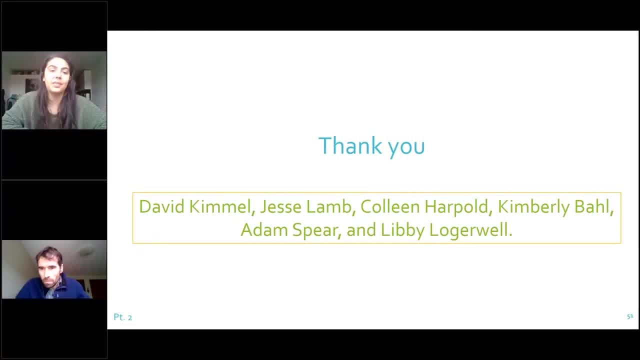 but it's a really good question. I want to keep adding on to my senior thesis with hopes of publishing it, so I'm gonna remember that question and make sure I answer it in my paper. there's another question from Jenna who says: thank you, at what depths are you? 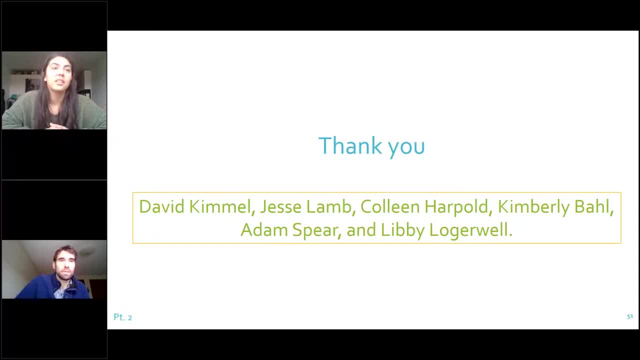 hoping to set up the autonomous surveys, assuming that's the the latest work you just talked about. yeah, I, I'm a professional when it comes to identifying the plankton that we're see and you know creating the algorithm, so I'm not exactly sure. I know that Calvin morning may be on the line as well as. 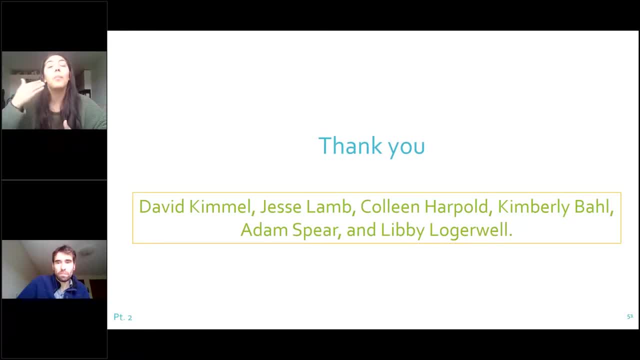 Dave Kimmel and they might have more details, but I'm hoping that my my assumption is that we're hoping to profile the entire water column, or as much as we can. all right, here's a question from Hassan Diana. could you elaborate about training data from machine learning algorithms that you mentioned? yeah, 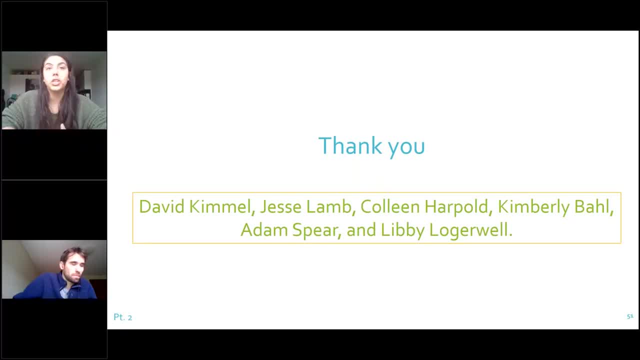 so I'm just getting started when it comes to machine learning using the image pro 10 software and because I'm just starting to load and generate image libraries on the system. the software is not able to automatically identify yet, but when I do good good in my software, if you notice in the picture that had the copepods that were highlighted. 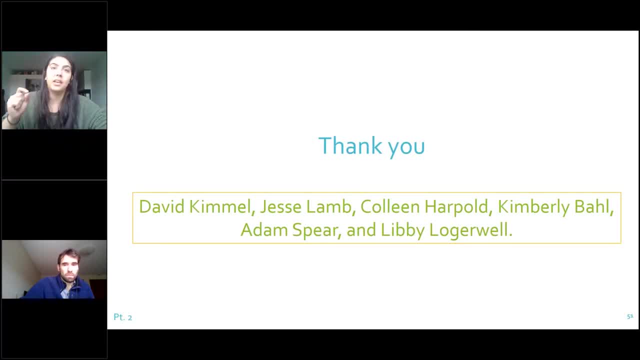 in blue when I highlight them. I have the option to set a classification and I tell the programmers this is a copepod. or I can even be more specific if I wanted to, but in the beginning I'm going to be really general, just to make sure that I can train the system. 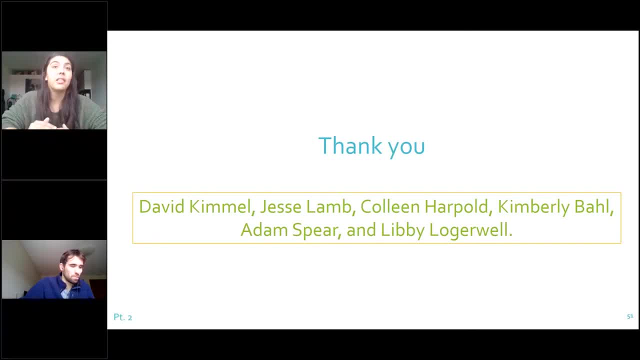 and I'll say this is a copepod or this is a euphosid and I set the class. so when it goes through I batch process. so I'll do a bunch of copepods all at one time and say: 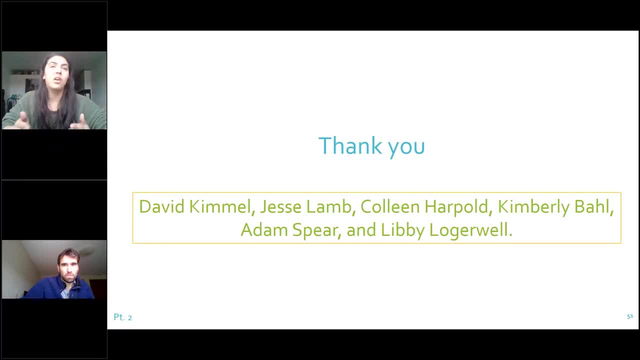 these are all copepods- and then all of the data that it spits out gets saved into a special learning file that the system software creates and once we get enough images loaded into it, the system will be able to learn and identify and reference back to those images that I 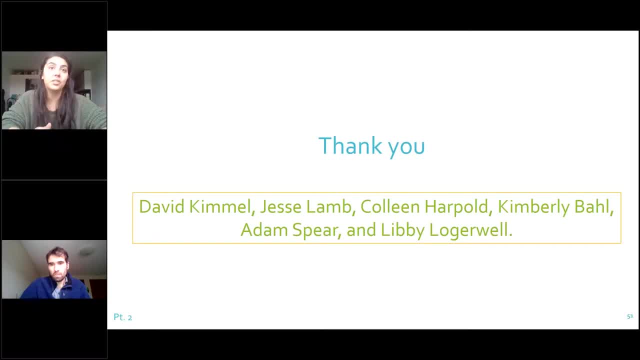 already provided to the system. so we need a lot of images to do this. with the AI and also even if we do collaborate with Google, the goal is we have to dump a lot of images in. So we're just in the beginning of generating these images, so I expect most of the next. 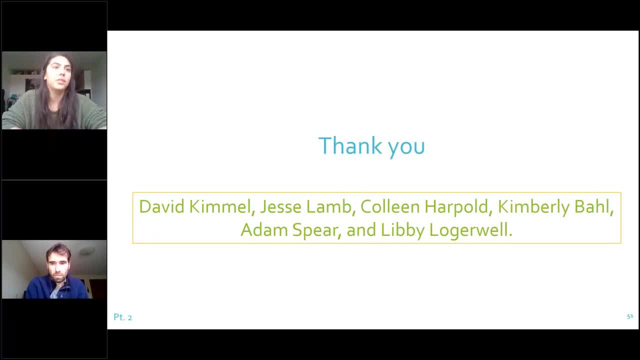 year to be making, just getting as many images as we can to train all the systems. All right, next question is from Patricia. I think, Yeah, you state that the temperature is warm and soup plankton may become smaller. However, do you think there will be an increased abundance of the soup plankton because of warming There? 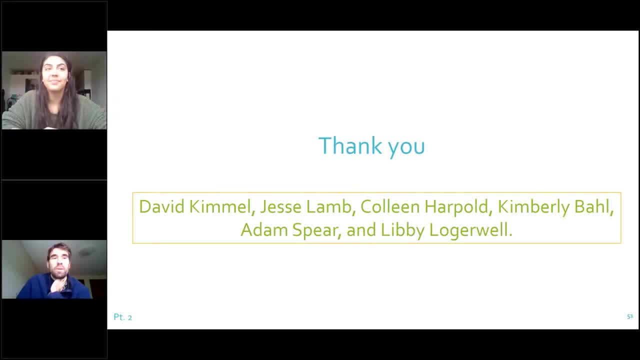 could be less lipids per individual because of the smaller size, but there may be an increase in numbers that could make up for that. That's a good point. yeah, I'm just trying to shift between my- I think of warming- and. 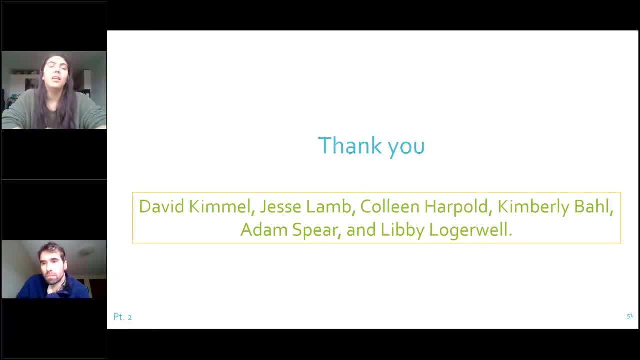 hypoxia, that's undergrad. so warming in the Bering Sea, there could be a change in abundance? It depends. let me think this one through: If it's warmer metabolic rates, they spend more time in the lower sizes. I think the higher metabolic rates might prevent them from growing and it might limit egg production, And so I'm not sure. Dave might have a little bit more insight about that. Yeah, that's a good question. Yeah, that's a really good question. So there's a paper out there that does spec. I should. 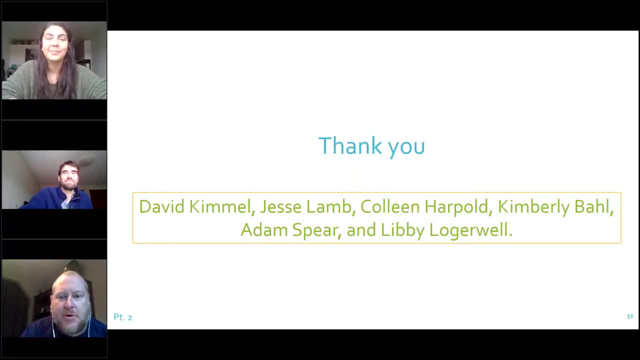 put my camera on. sorry, Sorry. Yeah, there's a paper out there that speculates is just that that there's going to be a shift in species composition and you may get more zooplankton, but they're smaller. my concern with that is that if they're different species, they don't accumulate. as much lipid. so they might have smaller amounts of lipid and there might be more of them, but they might be of different sizes, which affects the predator prey mass ratio and the trophic transfer. so, yeah, there's some competing hypotheses out there that there will be sort of increases in the overall abundance as it. 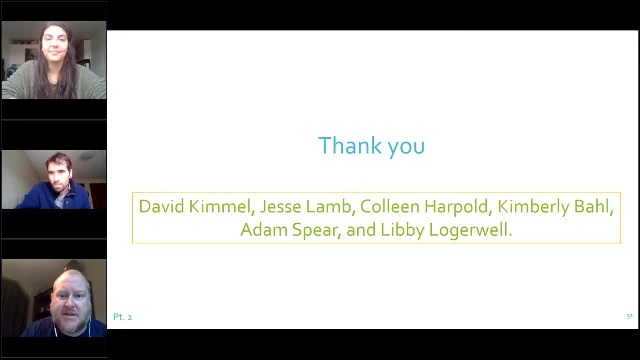 warms, but the I think you know for this ecosystem the type of species that does matter, because the fish have evolved to to use that as a particular food source. so yeah, great, great question. I'll shut up, sorry, no, thank you. thank you. next one's from Jim Overland who says: how strong are you bearing? 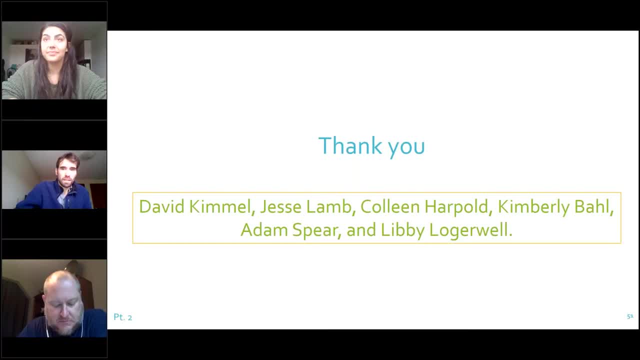 implications based on 2018 and 19, and I'm thinking that he really he's thinking about this very warm years and how that may have impacted us. so, plankton, do you know this yet? are you still looking at data when it comes to imaging? I don't know this yet. I haven't looked at data, but in 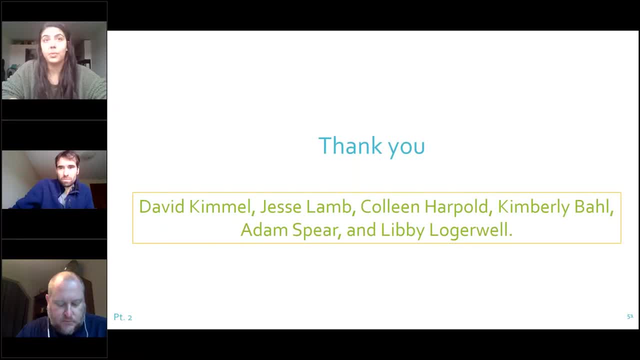 regards to Bruce, I haven't. I need to read more papers, and Dave might know a little bit more about that too, so we don't know yet, but we have zooplankton in hand that she's going to image and measure, so she just got started on that. 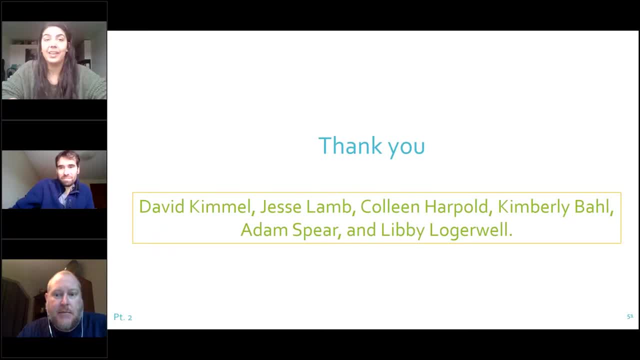 so we hope to have an answer on that relatively soon. I'm expecting to see some pretty dramatic size shifts. you know, even with a car show which is not a very big copepod, they saw about a hundred down the road and so we're kind of 100 micrometer change and that copepod is only about a millimeter in size. the 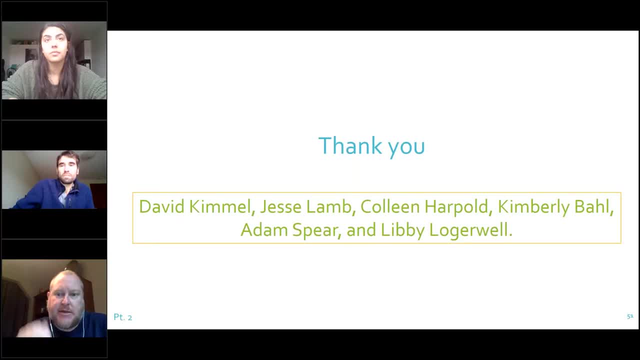 kalanis are triple to four times that. so I expect to see some of those changes. at least that's the hypothesis. yeah, Anna, just started measuring those. yeah, I started looking at 2012 to 2015 data. I want to say last week and my first, 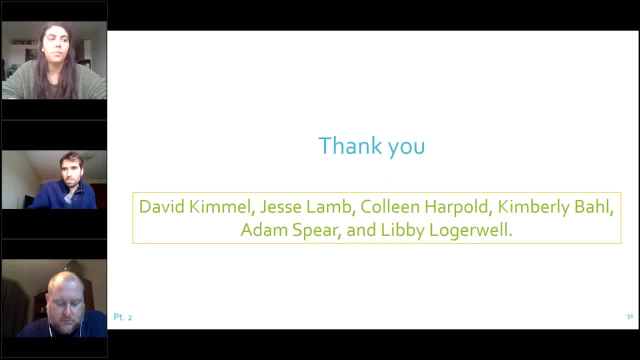 initial response was we not had a lot of and sex. we had a lot more females and we saw males relative to most of the years that we saw, and there were less adults- t5 copepods that were present, which was really, really surprising and, yeah, it kind of threw us for a loop. so I had to kind of recalibrate a little bit. 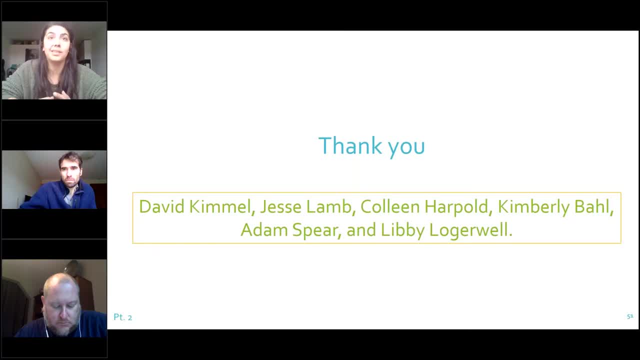 and figure out what to do when we have a really big shift. and we expected to see when it came to who we measure and who we image you all right, we're going to keep moving here. so Melanie says: in the Salish sea study you showed an o2 reading of 0.25 milligrams per liter. did you ever hit? 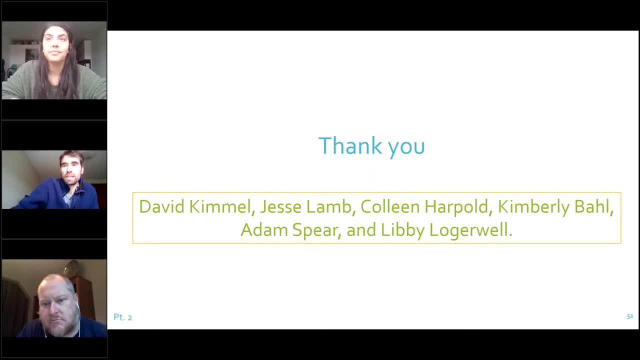 anything that low? also, did you approach that study with any info about metabolic differences between younger, smaller copepods and larger ones? so did I. the question: did I find any oxygen concentrations that low in relation to other conditions or another profile? I think I missed that part right there. um, I didn't expect oxygen. 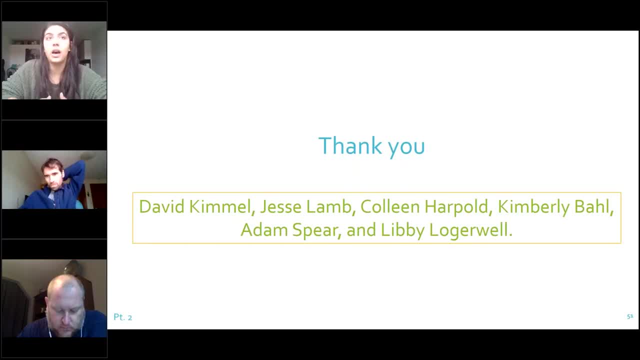 concentrations to get that low. but it's great that it did. there weren't really a lot of studies that kind of went that low in oxygen concentration, so it was really nice to kind of see that out. um, I did do research into the metabolic difference and I also did kind of look into species availability. I looked at 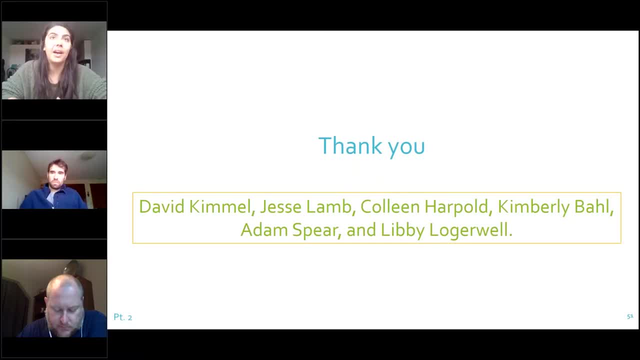 five different species of copepod that we found in that area and they all do have significantly different um, behavioral differences, size differences, um, and there is going to be implications in regards to the metabolic process. you know, with warmer waters and hypoxia, i expect there to be different behavior, um, that's something. 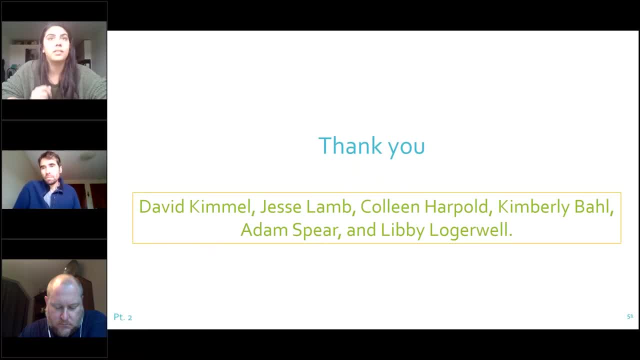 i didn't in my initial run on my senior thesis, but that is something that i plan on spending time on making sure that i have um a large kind of section, because it's really important, because the the implications of my data weren't very conclusive and it was kind of surprising and i i 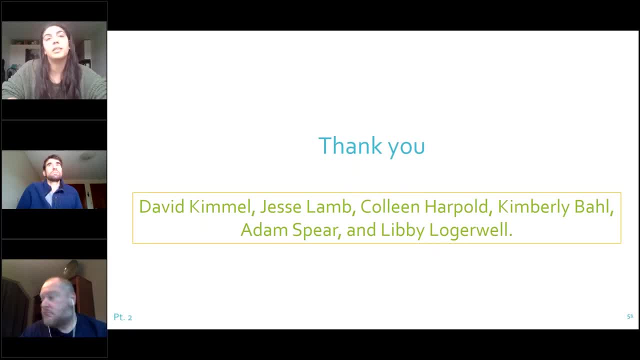 say: you know, that's probably what i'm going to have to rely on. next, i looked at body size and abundance. i need to now shift towards species abundance- exactly who's there and what the difference is between the metabolic rates. so that's a great question. next, 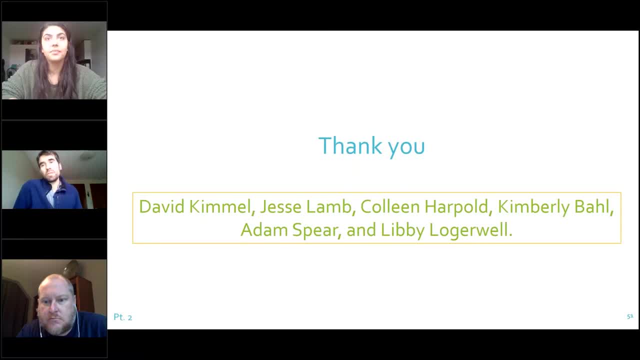 uh, a good question here from al herman. under warming, both zooplankton and fish may experience heightened metabolism. has reduced zooplankton could be due to both their own increased respiration or and heightened predation from fish- hungry fish. any thoughts on which will be more important? 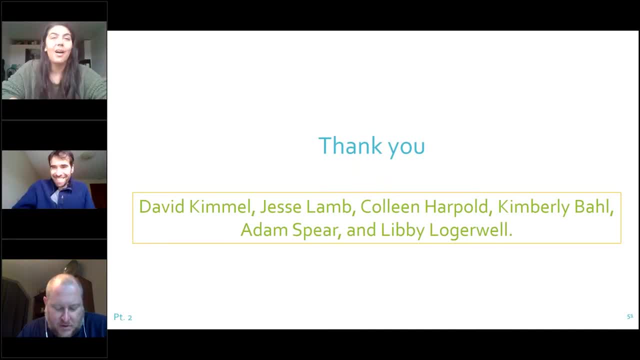 nice, easy one. um, no, i don't have any. i mean i'm a little biased, you know. i think you know what happens with the zooplankton- are the most important. i mean the. the trophic energy transfer is only 10 from each trophic level. so you know, if the 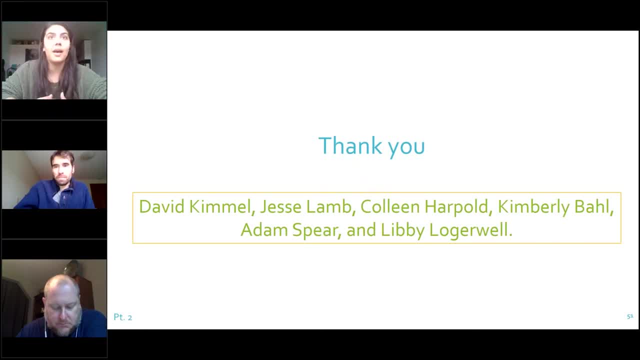 metabolic rates and the size of the cocoa pods are different. phytoplankton biomass is a little different. um, i expect it to be the- you know, just the main driver of what happens to the rest of them. so, even if, even if the fish are affected by it, i think that they may be affected by it, but i think 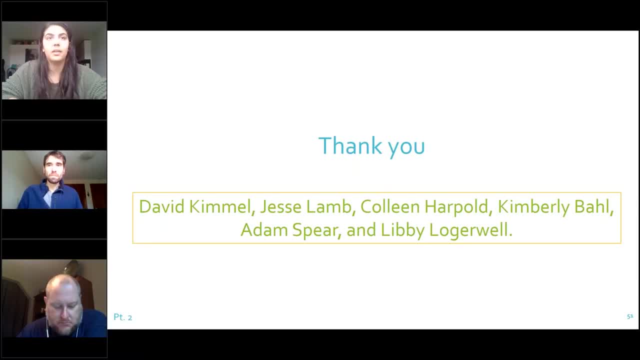 their biggest effect will be because of their food availability. i think the- yeah, a little bias. this is zooplankton. they're most important. and then let's see, here we have patricia saying production increases with temperature. i think that relates to the earlier uh discussion about uh lower sizes, but 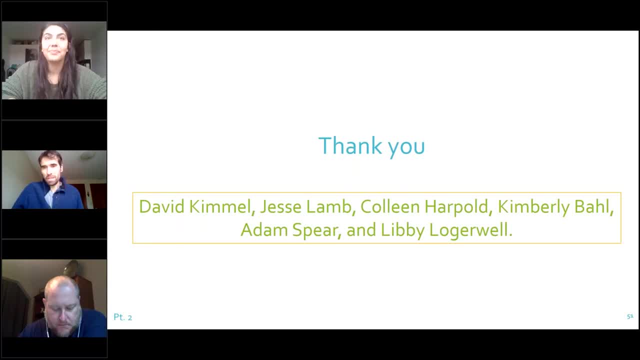 potentially higher production per individual. um, if you want to add anything to that, i think we kind of covered it. um, let's see another question from jenna. what kind of tech is on deck for the surveys? does the unit collect or take microscopic imagery? if it is capturing images to get finite, 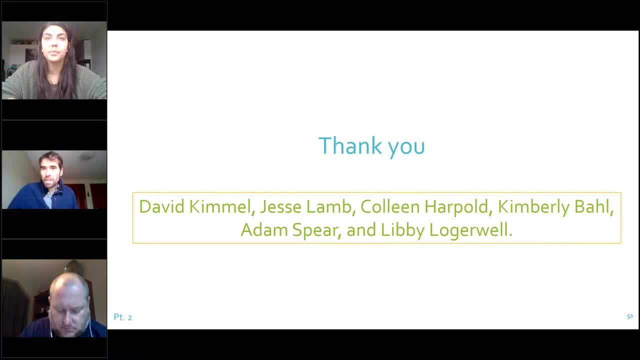 details. what onboard camera um technology does it have? i'm interested in learning more about the abilities capturing data in a highly productive area. yeah, um, well, um, the cpix is um something that is with calvin morty's group and pmel um i they're able to collect images. i'm not sure that they're microscopic i. 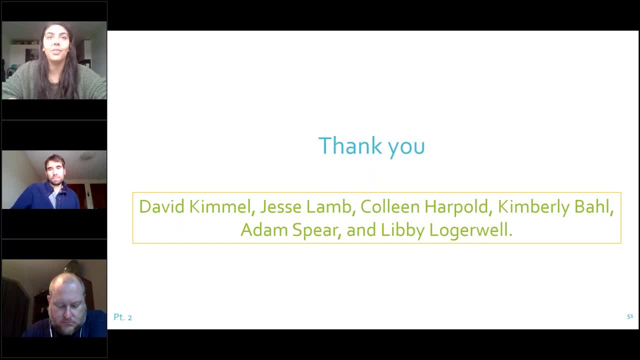 haven't seen it yet. um, i've just been able to, you know, kind of stalk around the websites, um, um, and get a good look at the aspects of the camera. um, but right now, when it comes to in-situ work, that's the camera that we have working on, and then 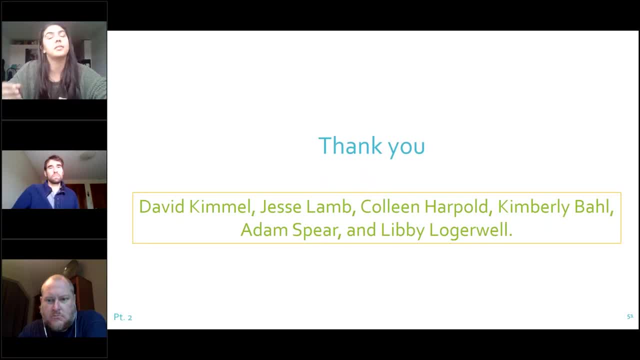 we plan to pull on board and take microscopic pictures on board. so whatever we catch in our nets and look at under the microscope while we're on board, um, we'll use microscope for that, um, so, yeah, it's really exciting. i'm really excited about it too. definitely reach. 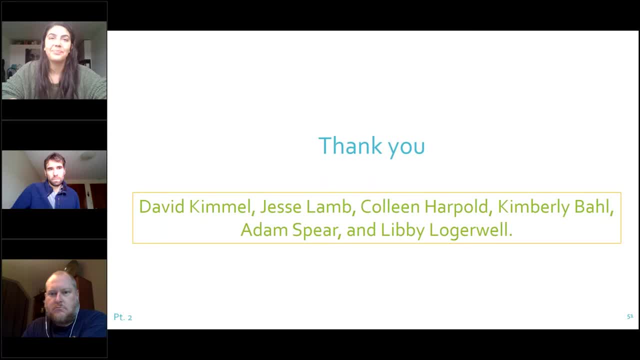 out to to dave and calvin and bill. they're gonna probably talk to you about it more. yeah, i can. i can add to that that- noah, I always get the name wrong- but basically similar type of approach to take phytoplankton images, which I think will also be tested next year, a phyto 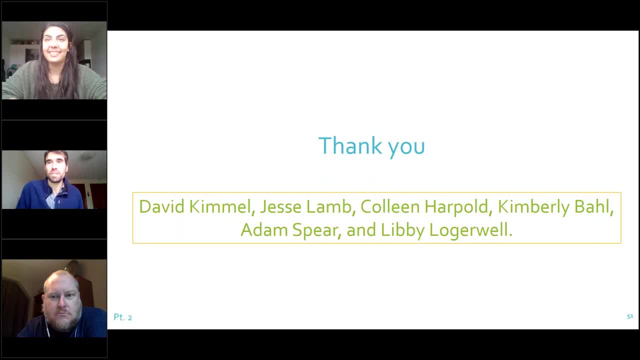 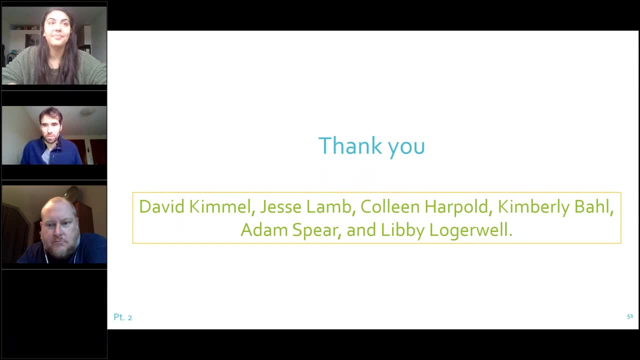 something bot or something like that. Jeanette Gann- I don't know if she's on- is sort of the expert on that, so let's see. moving on, Patricia says thanks for presenting interesting work. I do zooplankton work in the Great Lakes, so I appreciate all the fellow zooplankton nerds. thank you. 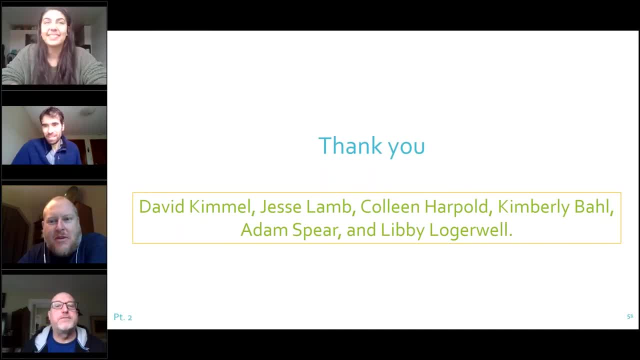 I was just gonna mention that the camera should be here in time for the spring mooring cruise, so we'll put it on the CTV and have it collect images while we're doing the net samples and hopefully that all works and then we will have it on the fall cruise through the Bering Sea up through the Arctic. 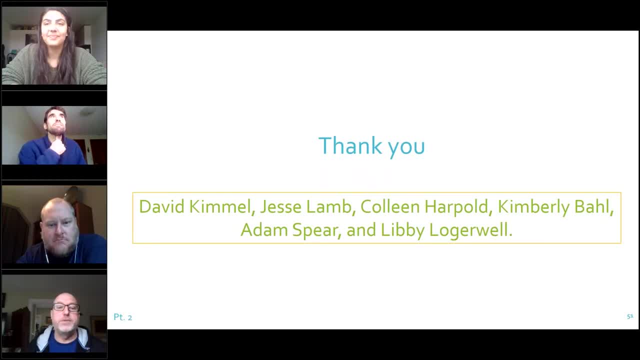 doing the same thing on the CTV. if everything looks good, we'll be thinking about other applications on on moorings. so we'll see how that goes. Dave, you have anything else to add to that? no, I'm just that. yeah, it's coming. that should be here in January. we're gonna put it through its paces in Puget. 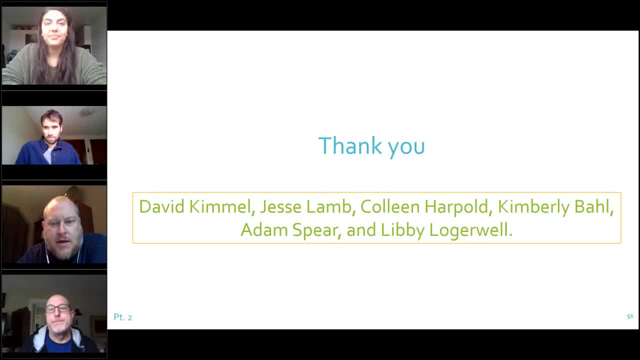 Sound, and and the other thing is we're really relying on Poland to produce annotated images. we had a question earlier about artificial intelligence. you know, one of the main rate limiting steps there is getting training data set. so what we're doing with our colleagues as Poland is they're producing the 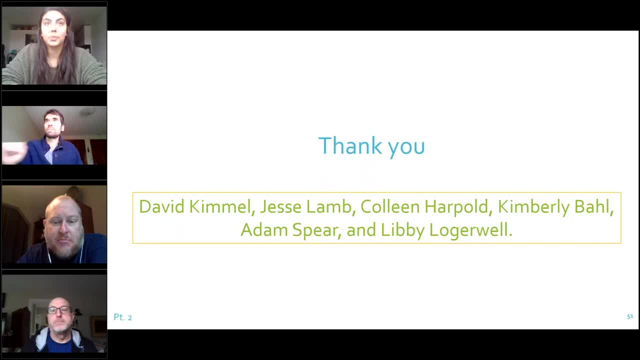 images that are already sorted in, annotate And hopefully building up that library so we can produce artificial intelligence algorithms that are a little bit more annotated, because many of these software limitations are due to the fact that training sets are just really laborious to produce. So we're hoping to get by that by helping with our colleagues in Poland. So we're really excited to converge all of this different activities and technology that Deanna is sitting at the nexus of to help us advance this science. 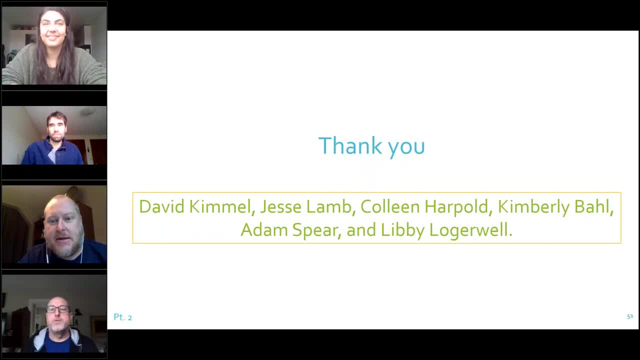 So we're very excited to get out in the field next year and do some of this. And will either of you be on the spring morning cruise? Do you have plans for that or is there still COVID concerns? So I have indicated that I will. 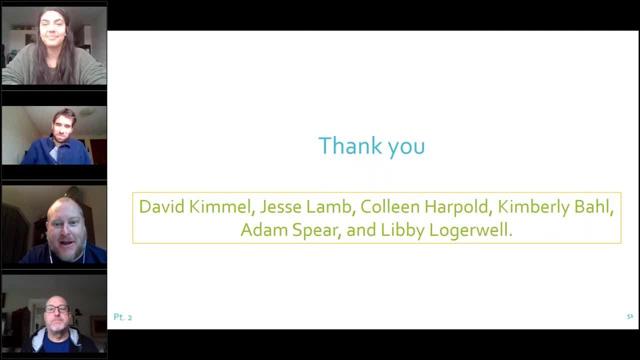 I would like to go on the cruises where the camera is deployed as the main dude to help. Okay, Well, we'll see how that works. Yeah, We're going to try, Calvin, to get it working with Jeff and I over the winter. 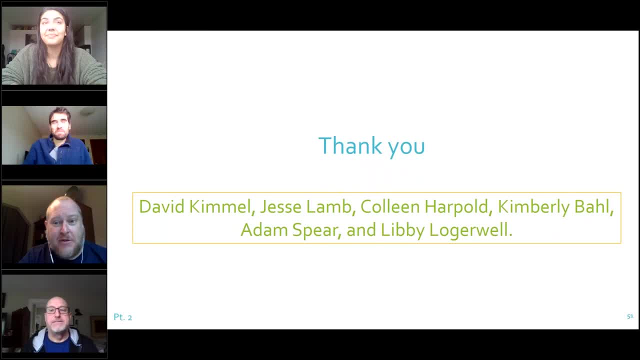 And then Deanna is going to be involved with that with us and make sure that we have two folks that know inside and out how to work with the camera and the software in the field. Meaning just some dock deployments, Yep, Dock deployments, Maybe a little. 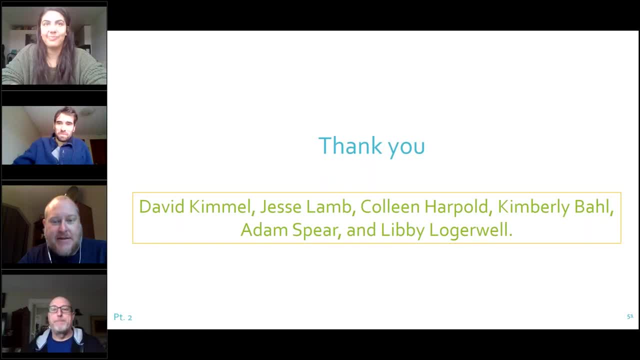 Small boat action, if we can try it, to get this thing in the water and try to take some images. And Julie Keister is on the line somewhere and she's got some cool images of Puget Sound, plankton. So if we get some cool pictures there, we might be able to compare to some of the work that she's done. 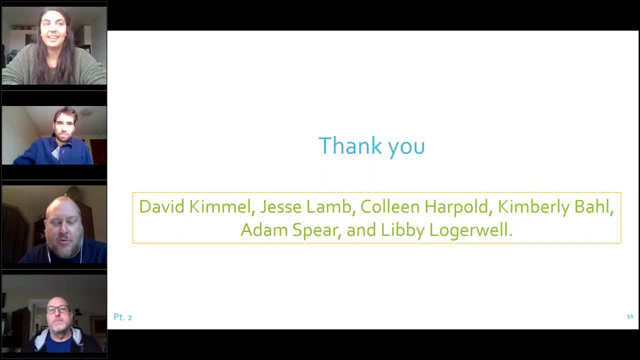 So we're- yeah, we're- very excited about this and hoping to have folks in the field that are going to be working with this stuff closely with you, Cal. And then we also had the Google team actually come to PMEL and give us a shot. 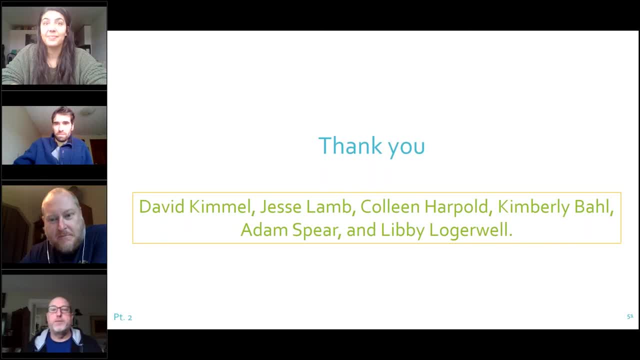 Show and tell of their AI system. It's quite impressive, Yeah, and we need, you know, we just need images. We need images that are annotated to begin training the system, And that's really the yeah, that's really the part we're looking forward to. 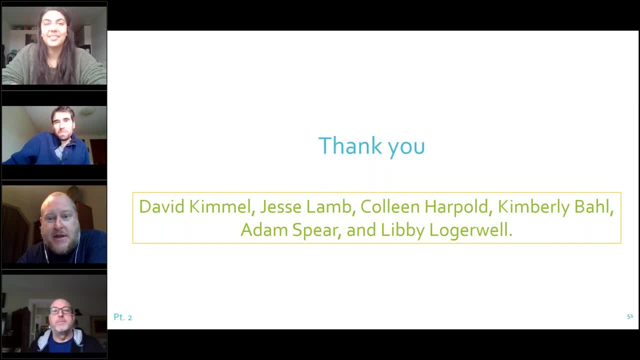 So Deanna's been really instrumental in moving this needle on this. We've been sort of talking about this for a while, but we haven't had people in here to work on it And Deanna's just really jumped right in and grabbed the bull by the horn.